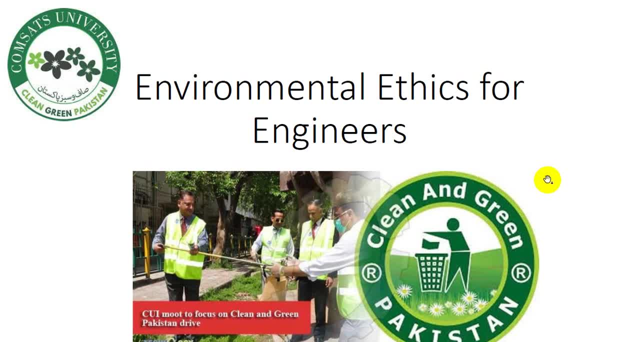 Assalamualaikum, students, This is your week two for engineering and professionalism course. Just like last week, we were discussing safety and health and ethics about safety and health, This week we will be covering starting the second part of the course. As you know, there are three parts of the course. First one is related to ethics. Second is related to ethics. 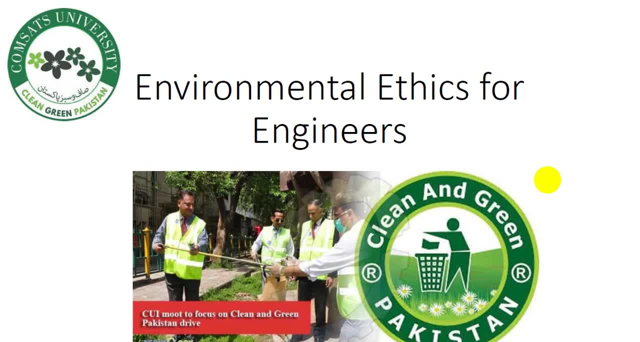 Environmental ethics and sustainability. So today, in the first lecture, we will be talking about environmental ethics for engineers. So what role engineers can play in the environment? First of all, what is environmental ethics and how engineers can improve environment and use sustainable development. Before we start, I want you to realize this: that this is an important part of the course. Let me just 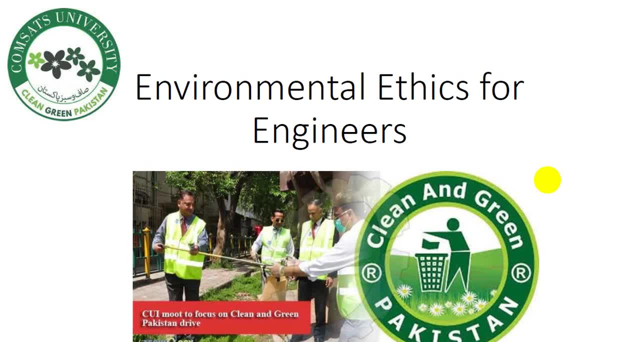 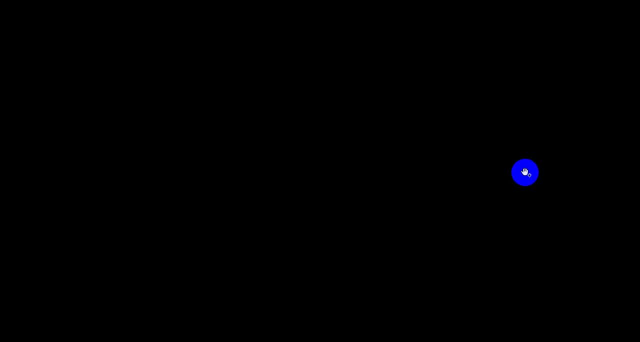 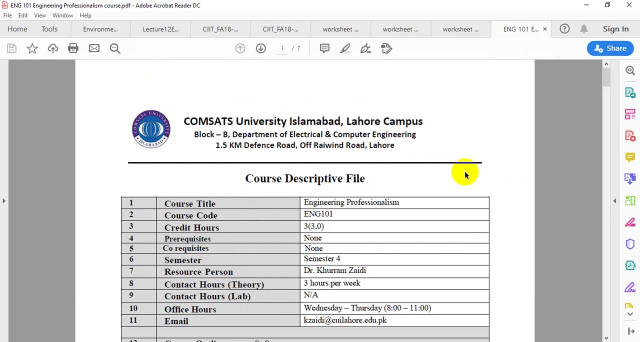 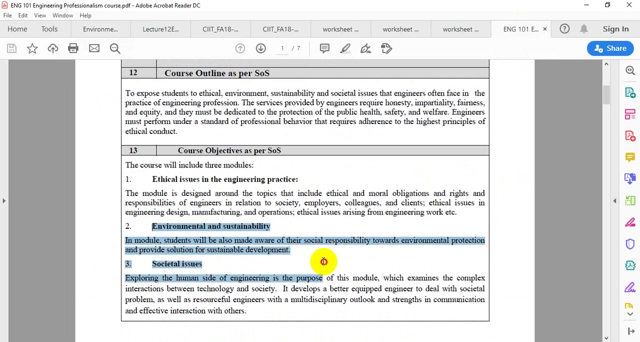 recap our CDF: As you know in our CDF, let me just go back and open CDF for this course. So if you just open CDF, which is on your see online, you can see that environmental and sustainability- This is the second part of your course, One of the course objectives. We have already covered the ethical issues in engineering practice. 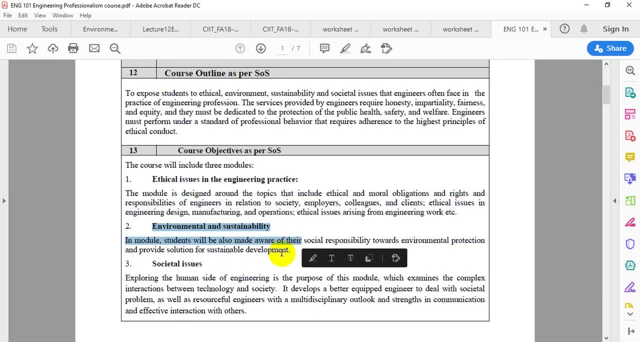 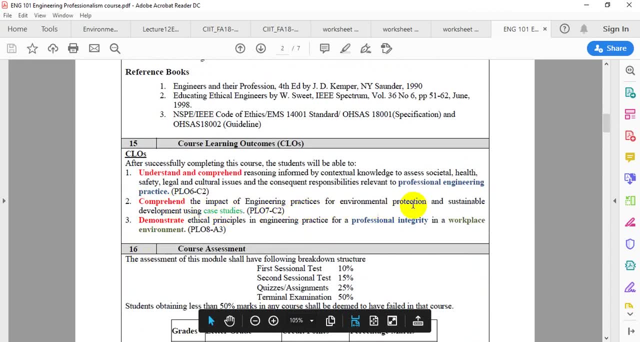 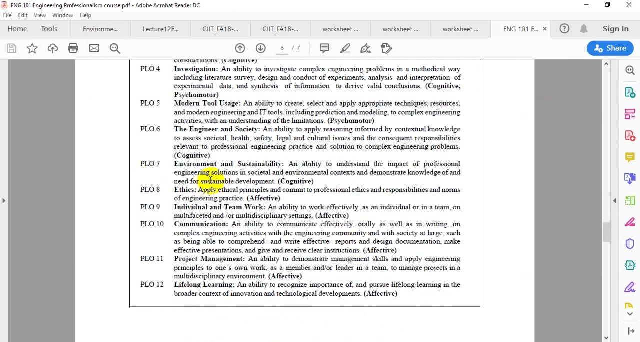 So we are now on to the second part and even our CLO2 in your OBE: comprehend the impact of engineering practices for environmental protection and sustainable development using case study. So this is what we're going to cover now. See your CLO2, which is mapped into CLO7 and, if you go, remember your CLO7. your CLO7 is environment and sustainability and ability to understand the impact of professional engineering solutions. 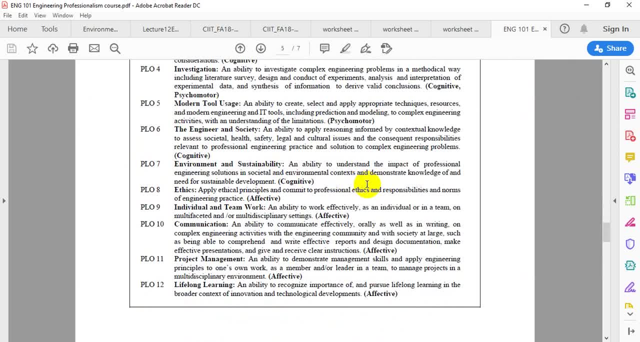 So let me follow up. So our next topic to cover is sustainability, and sustainability and inclusion. Here we are showing you a perfect example of a concept and the way it is accentuated. TIM Ezch estudied it. study it In societal and environmental context段 caped down: 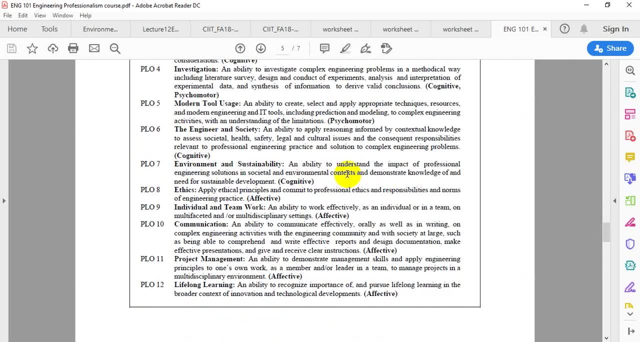 And demonstrate knowledge of and need for sustainable development. ________ scholarship photos. So the next elbow this week in the next week, these 2 weeks will be covering environmental ethics and sustainability. Ignition that sacar m oxide, Any, is what we'll go through. so this is important part. you must all also remember that you know from your 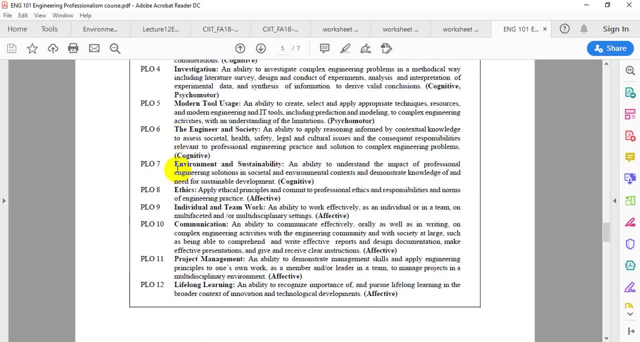 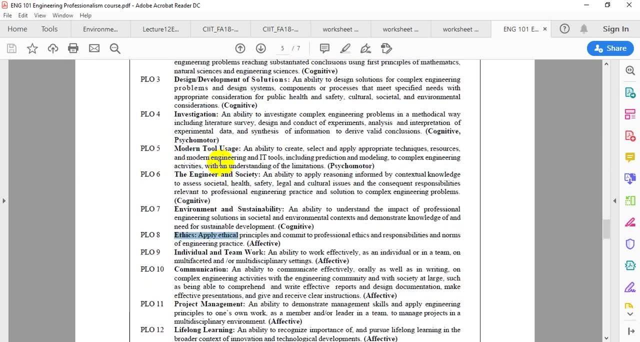 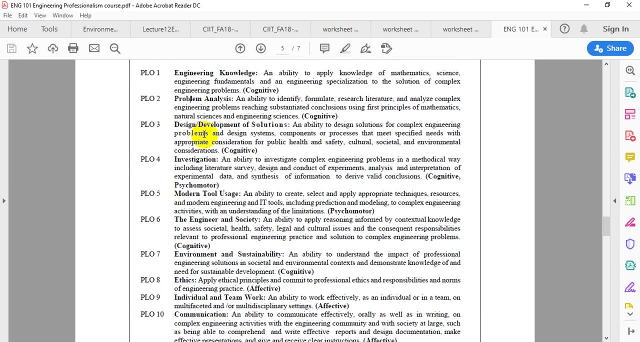 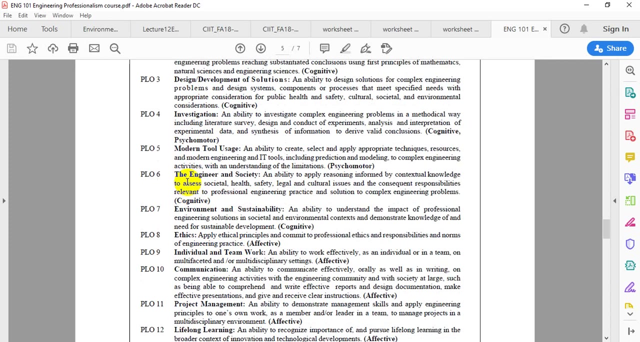 12 plos, uh. these plos like environmental and sustainability, ethics- these two are not covered in every course, like you know. the first five or six plos that you nearly every course covers. these plos like engineering, knowledge, problem analysis, uh, development solutions, investigation, modern. but these three plos are specific to this course and that's why this course was added. 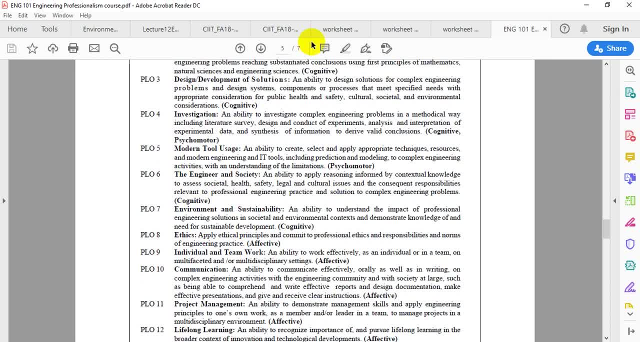 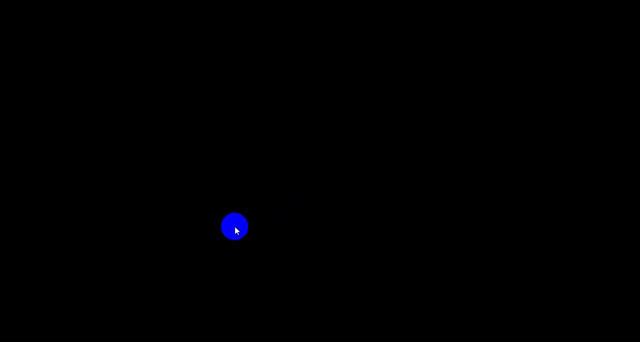 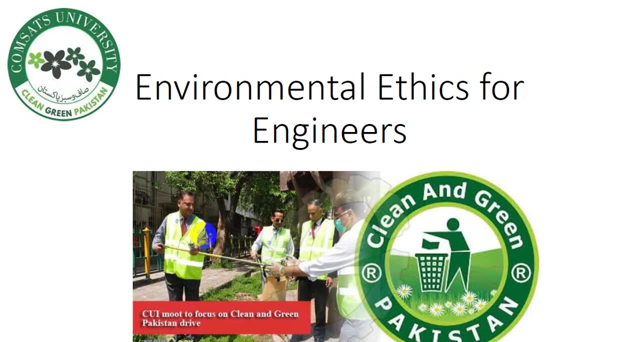 so this is important- that you must attain, uh, the required level. so let's go back to our uh in my environmental ethics: what is environmental ethics and what are the basics? so this is. let me just emphasize on the fact that comsats from last year has also started. 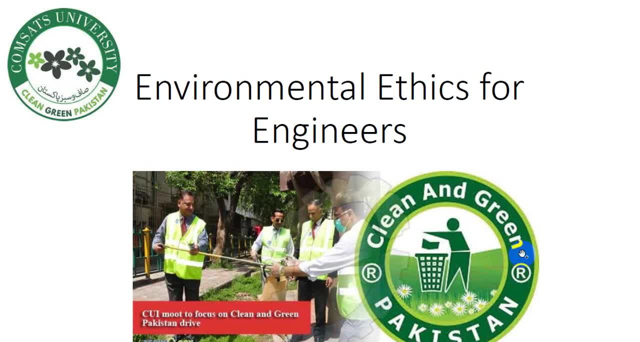 a scheme called clean and green pakistan. you know it's actively playing its role uh sa for subs pakistan. you can see the logo of conversation ministry, our rector uh dr professor, dr rahil kamar. he started this uh in islamabad. see why you want to focus on clean and green. 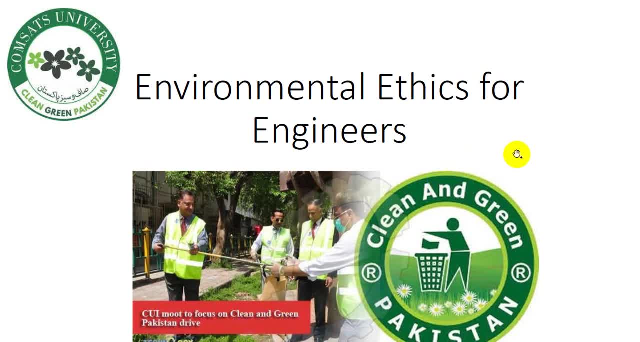 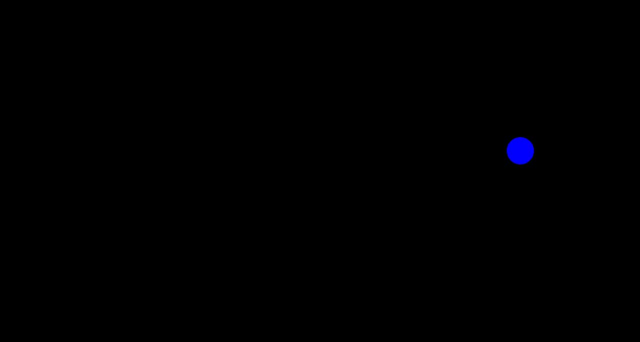 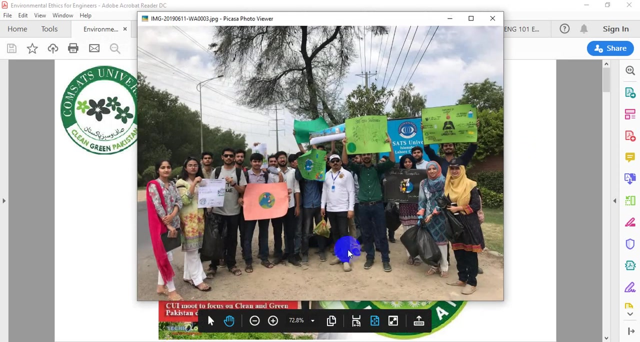 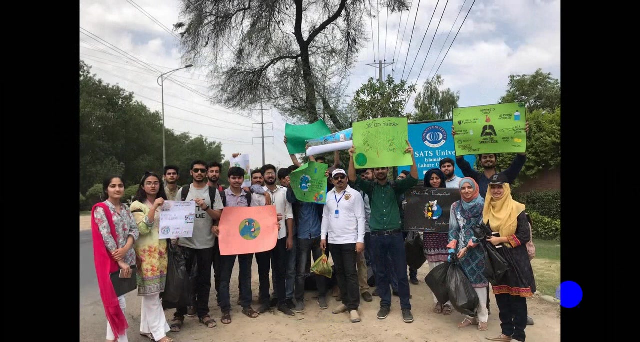 pakistan drive, where a cleaning drive was achieved in islam. following on his footsteps, i also arranged a clean and green drive last year with my previous students in the previous course. uh, let me just show you quickly, show you some pictures just to motivate you guys. so, if you can see, yeah, so if you can see that this was our clean and green drive, you can see me in the 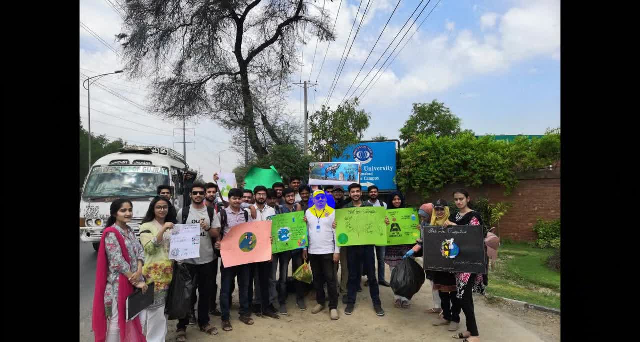 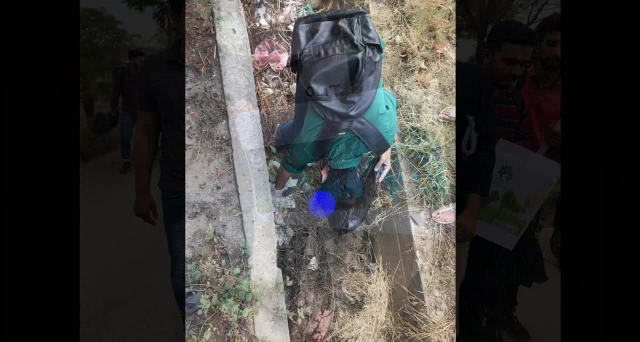 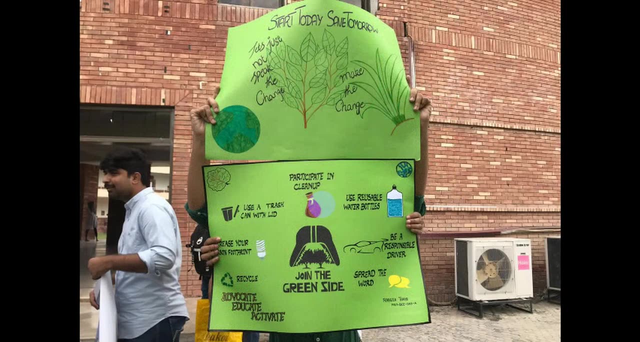 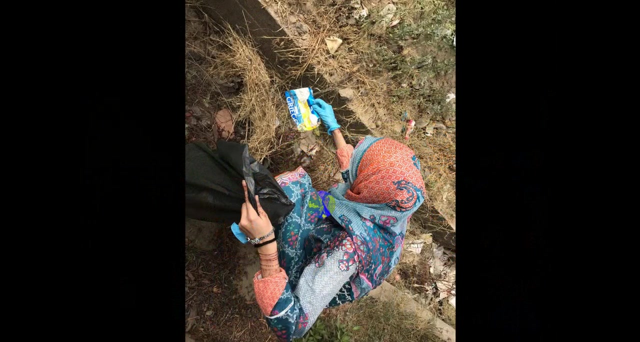 center there are some students. these are fa17 students- you're seeing one year senior students. so we arranged this drive, uh, from the new lecture theaters, from the end block to the defense road and the other students are doing the cleaning there. some plastic bottles, plastic bags, with all of them had made very lovely, beautiful chart papers, uh to display uh the drive was from. 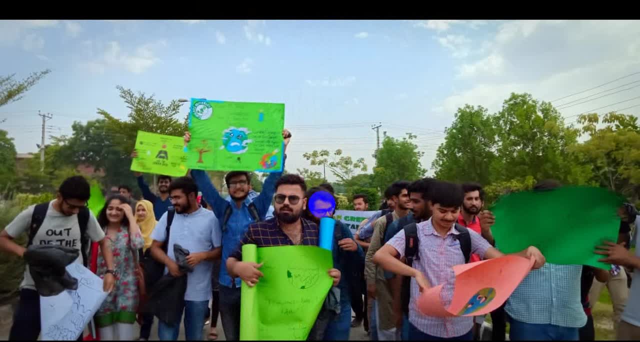 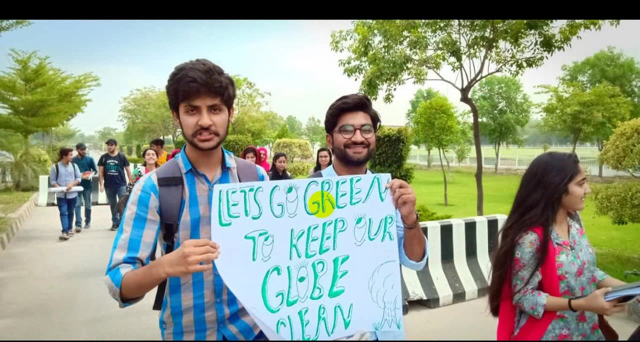 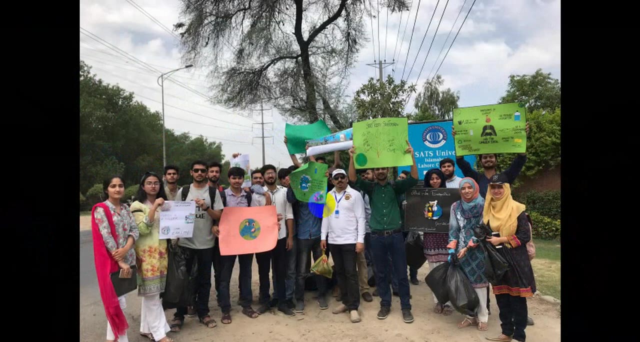 the new lecture theaters to the defense road. students actively participate. each student brought a uh bag- you can see that black bag at the in the background- so they had to fill up this bag and throw it in the dustbin. so, uh, it was very nice effort. unfortunately, this year we won't be able to. 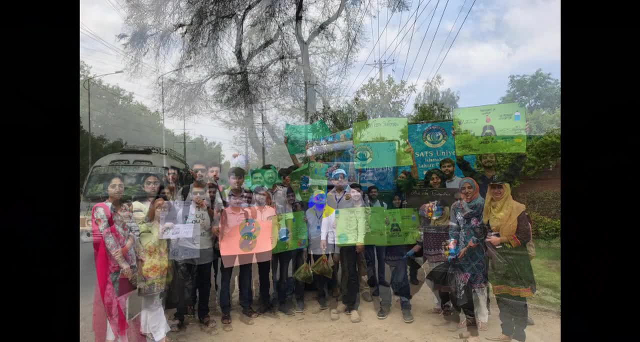 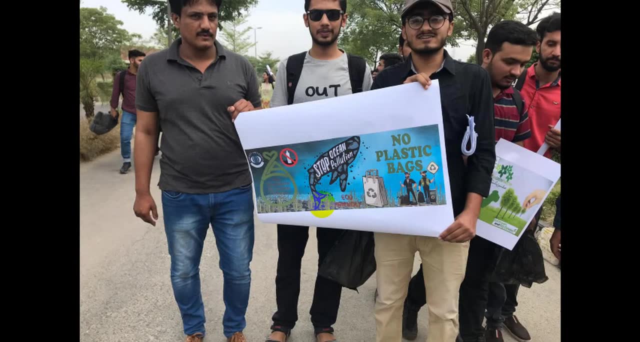 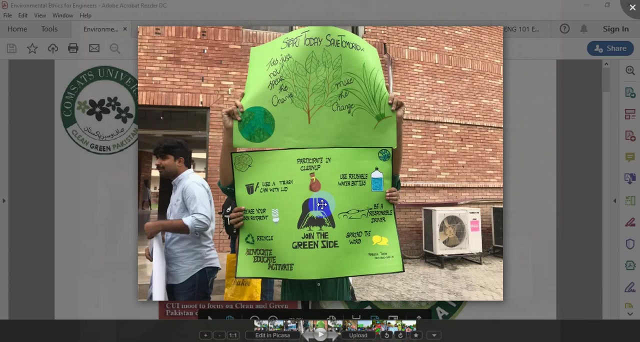 to do it because of the COVID-19 situation, but if it wasn't for that, we would would have surely arranged this clean and green drive this year. I had also planned to plant some trees, but unfortunately we couldn't do it, so but it's okay, we can still do it. I have given. I'll be probably giving you some. 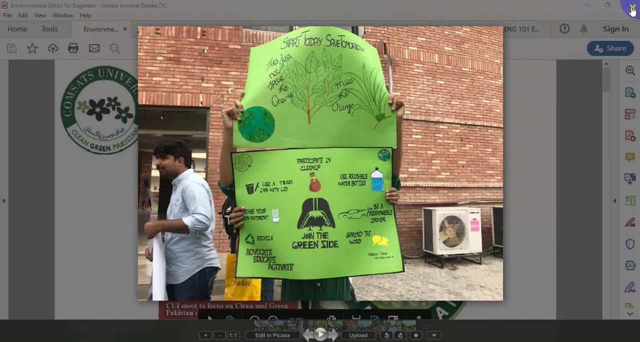 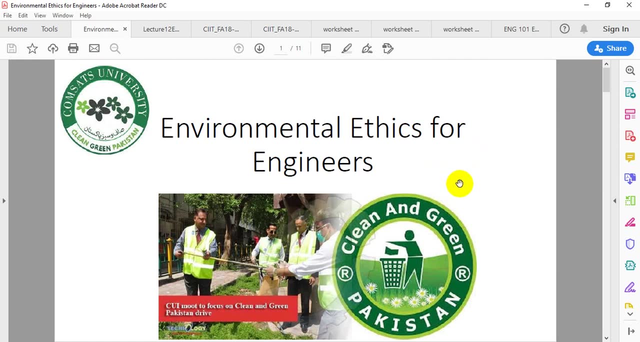 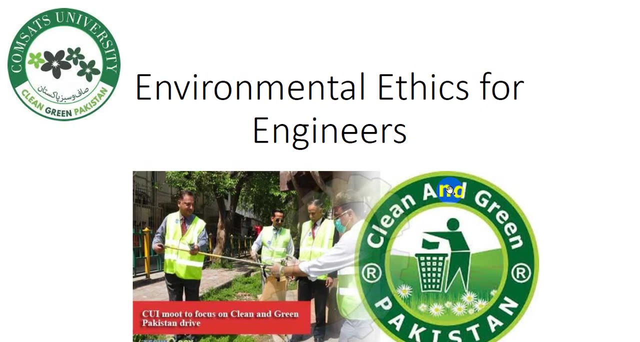 assignments that you can still do this at your home and do it in your community. so this would be part of your assignment, the project assignment that I will be giving you, that I will discuss next week. so let's get back to our lecture for today. so this was just for the motivation and so that you can. 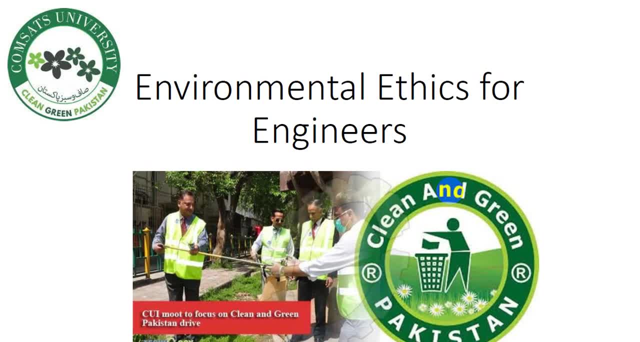 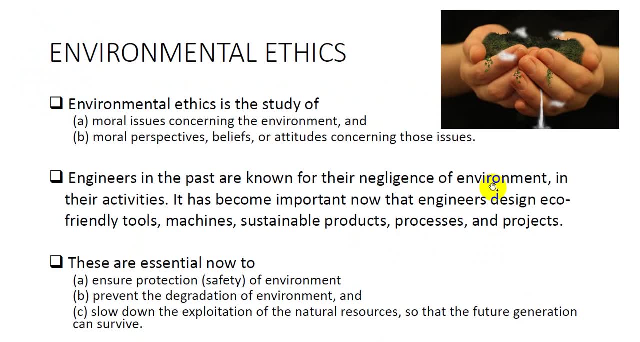 understand why it is important, and then I will also discuss what role you, as engineer, can play. environmental ethics for engineers. okay, so first of all, what is environmental ethics? environmental ethics is the study of moral issues concerning the environment and moral perspectives, beliefs or attitudes concerning those issues. so 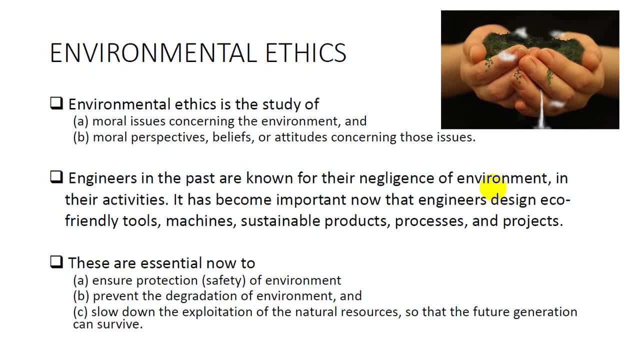 it's basically the issues concerning the environment. it's very simple. i mean, it's not a new thing, you all know it. you all know the issues with environment. okay, so it's just your perspective, your belief and your attitude towards it. so, if that attitude is good, your belief and 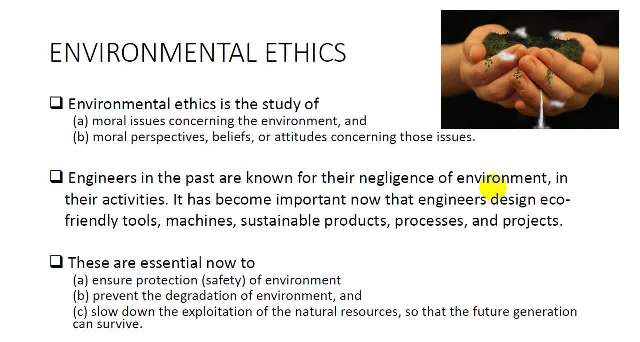 perspective that it is important. then this becomes environmental ethics. okay, so simple as that. so, as a human being, as an educated human being, as a muslim- because i will be quoting some examples from quran and hadith- this becomes our objective: that environmental ethics is very important, and 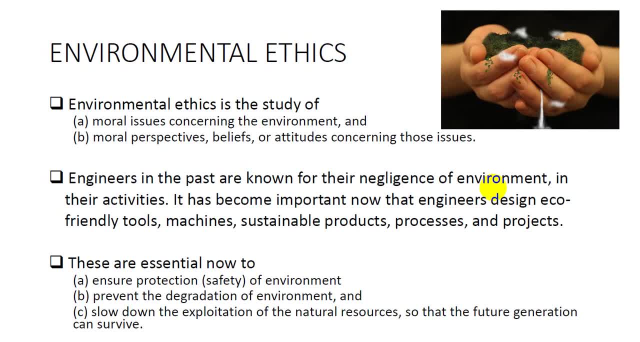 it plays an important part in our life- 50 percent. it is part of our iman and part of our religion. okay so? so engineers in the past are known for their negligence of environment in the activities. it has become important now that engineers design eco-friendly tools, machines, sustainable products. 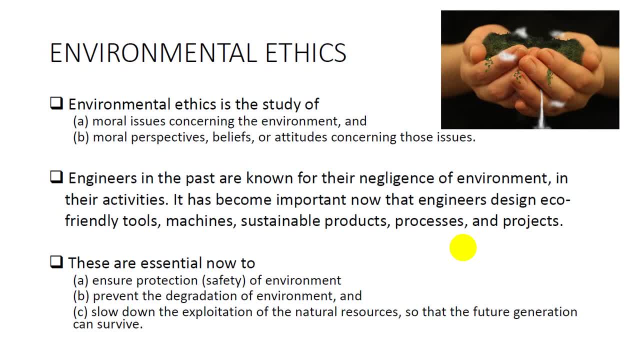 processes and projects. so in the beginning- you know the 19th century, when it was the era of the coal engines and industrial age- engineers were just thinking about making new products, making engines, making things for the human being, but in that era they were not able to do that. so engineers in the past are known for their negligence of environment. 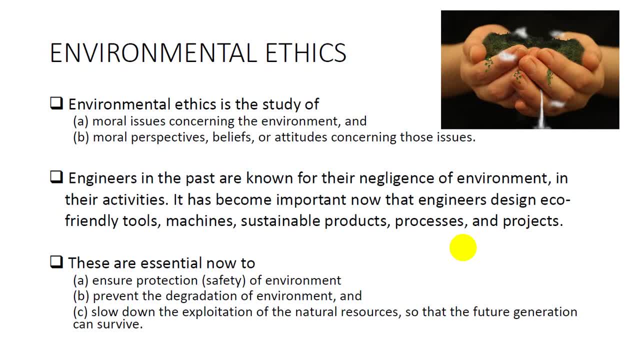 really neglected the environment part of it, but now, in very soon, it became clear that how we had polluted the whole planet, and it is an important part. so now each and every product that is being designed by engineers, the it is very important to consider the environmental and sustainable aspects. 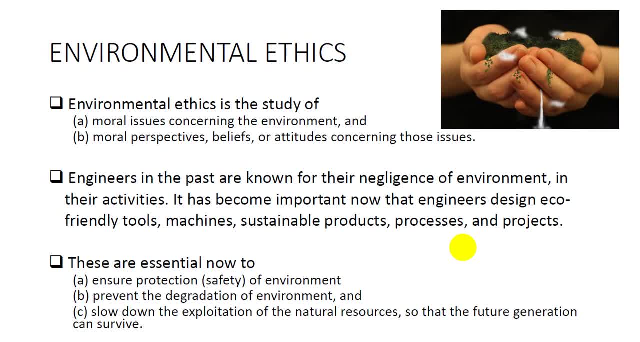 of it. okay, so i hope you understand this- that now, whenever you do, when you, when you graduate from here, you go into the industry, anything you design, anything you make, you must consider the environment and the environmental ethics part of that design. okay, these are essential now to ensure protection. 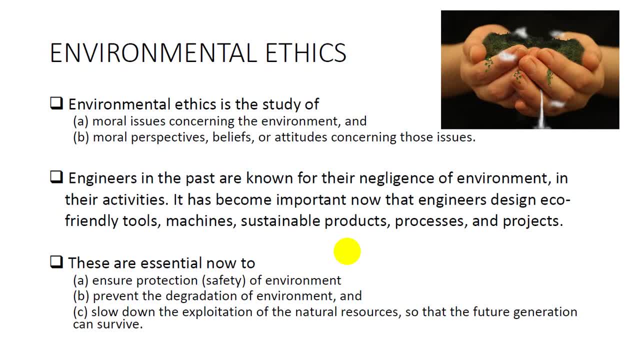 safety of environment, prevent the degradation of environment and slow down the exploitation of the natural resources so that the future generation can survive. so these three have become the important objectives, the essential part of every engineer. so whenever you go industry, probably your. the industry is being regulated by the government and the government ensures that each industry is being 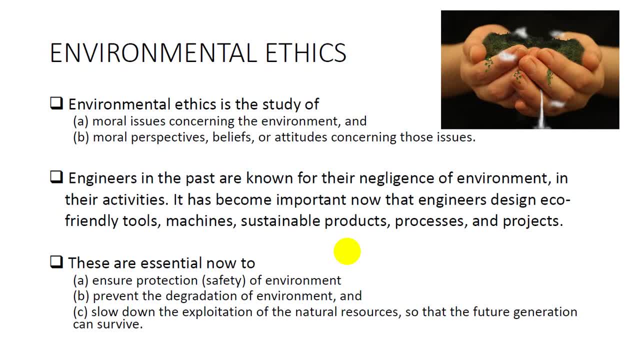 follows these parts, especially in the western world. in the modern world, they're very strict about it, although in our developing, in in the developing nations such as our country, people are now also now realizing our prime minister, imran khan. he's also emphasized that we should worry about the environment and 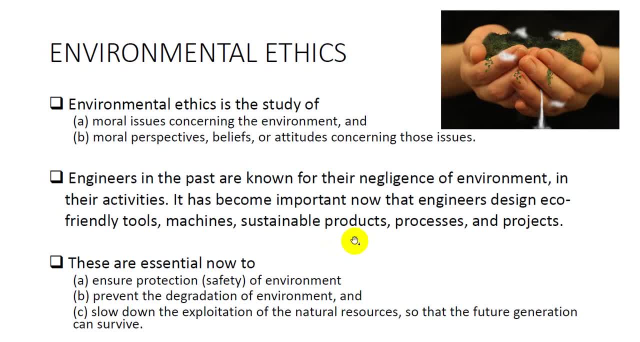 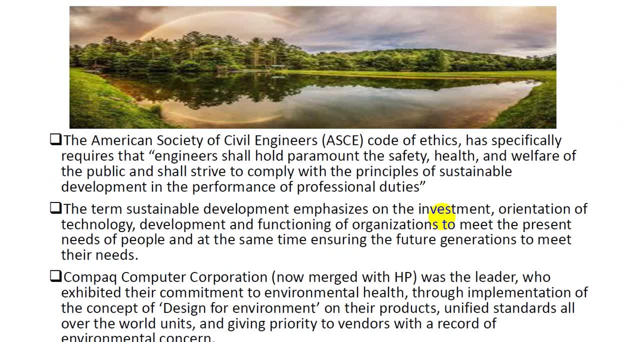 design things that can improve the environment. okay, the american society of civil engineers that we had already- we know what is asce we discussed in previous lectures- code of ethics has specifically requires that engineers shall hold paramount the safety, health and welfare of the public and shall strive to 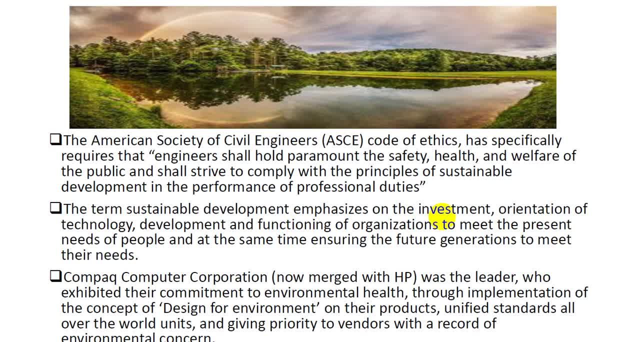 comply with the principles of sustainable development in the performance of professional duties. so it is the code all those civil engineers. it is their code, it is part of them. what they have to do is that they have to comply with the principles of sustainable development. okay, the term sustainable development emphasizes on the investment orientation of technology. 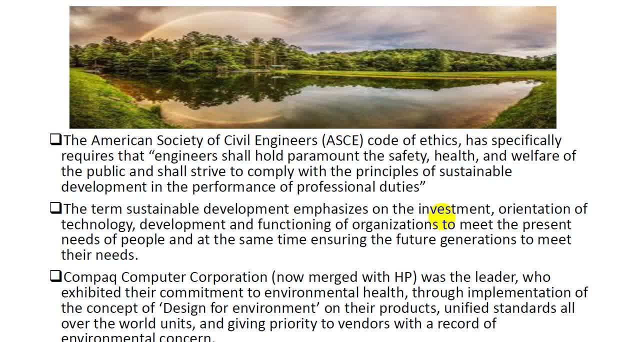 development and functioning of organizations to meet the present needs of people and, at the same time, ensuring the future generations to meet their needs. so environmental ethics is what we do now- okay, and then sustainable development. sustainability is that whatever we do now affects our future generations. so if we protect the environment now, if we protect the natural, 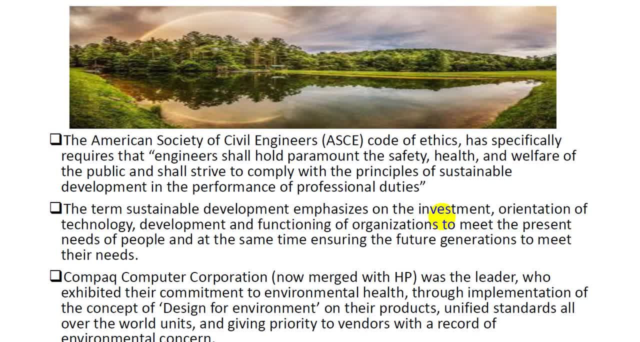 resources now, then our future generations can sustain our future generations and we can sustain much better and have a much better life. so what we do today, we will reap, we shall reap tomorrow. okay, compact computer corporation. you know, compact, uh, just like ibm, this is a computer corporation now. 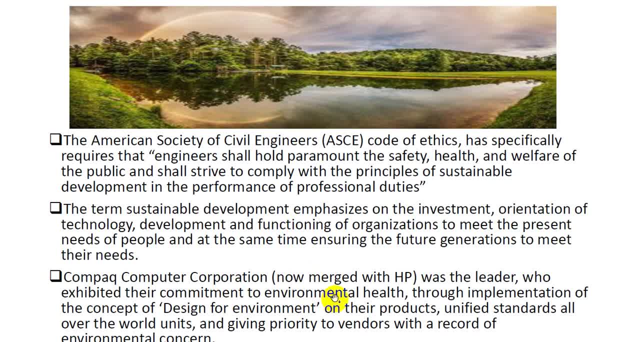 merged with hp, it is now renowned as hp. uh aholid packard was the leader who exhibited their commitment to environmental health through implementation of the concept of design for environment. so they had this concept, they had this tagline. you know that, whatever they're going to, 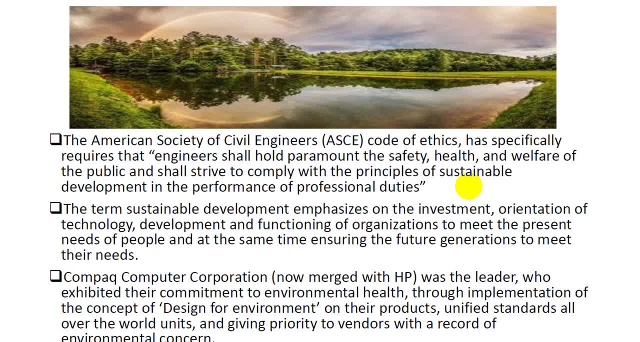 design. they're going to design for the environment. okay, whether it's expensive or not or whatever, they have to go through, they would need to go through, but they would design for the environment through implementation of the concept of design for the environment on their products, unified standards all over the world units and giving priority to vendors with a record of. 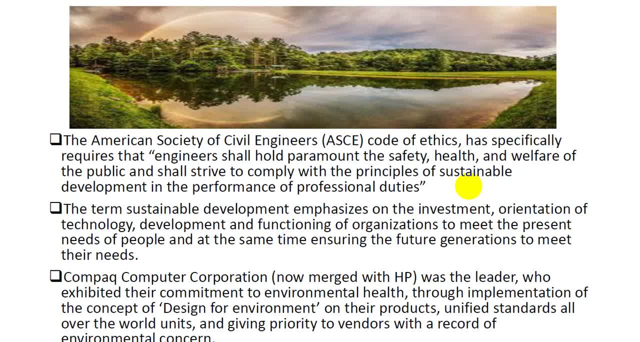 environmental concerns. so this is how you can ensure that whenever you need uh to engage some vendors, you further. your first priority should be that whether they uh uh, those vendors have a record of environmental concern or not. so this is how you can ensure in environment and sustainability. 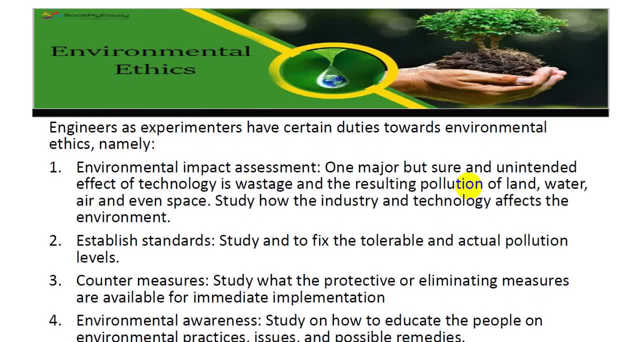 okay, engineers, as experimenters, have certain duties towards environmental ethics, namely environmental impact assessment. one major but sure and unintended effect of technology is wastage and the resulting pollution of land, water and air, and even space, because you know, just recently i was reading an article about space junk. i mean, you can't see it from here? 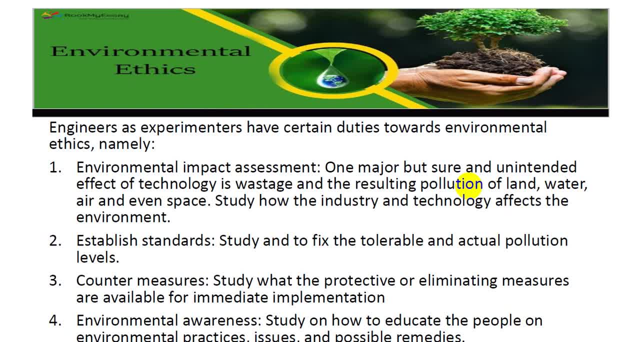 but if you go in space, there's a hell lot of pollution in space because, due to those satellites and those things that sent up there and it, there is no dustbin there, so it's just roaming around there, just circulating around there. so this now it has. 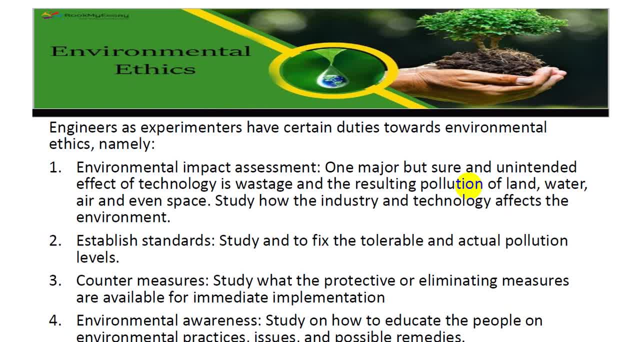 become a huge problem- the space junk- okay, so we'll talk about that later. study how the industry and the technology affects the environment. so number one is: is environmental impact assessment, okay. number two: establish standards study and to fix the tolerable and actual pollution levels- okay. so this is these. what kind of 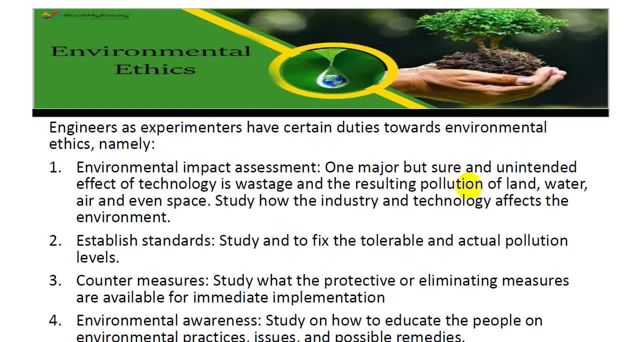 standards you will establish for any product design. number three: counter measures. study what the protective or eliminating measures are available for immediate implementation. so this is accountable. but but uh, we had already done what uh, pollution, we had already contributed to how we can now do counter measure number four: environmental awareness. now, this course is one part of 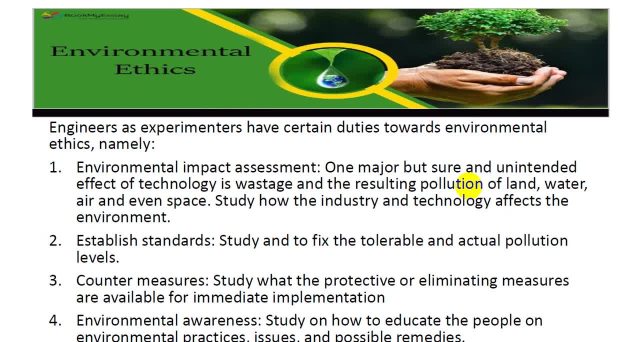 environmental awareness. then when you talk to as an educated engineer, when you talk to your friends, colleagues, your uh parents at home or your other family members, you can tell them what is environmental ethics and how, why it is important. so you can just spread the awareness through different social media. 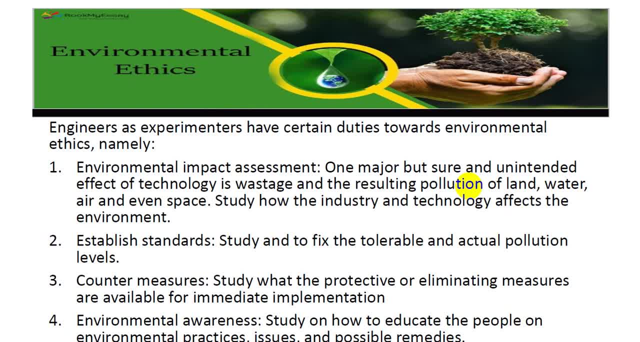 campaigns as well, whenever most of you are on social media like facebook and whatsapp groups, so you can spread awareness regarding environmental. we will do one of the uh this because now most of you are at home and it's very hard to go outside and do the clean and green drive just like we did last time. that was one part of the 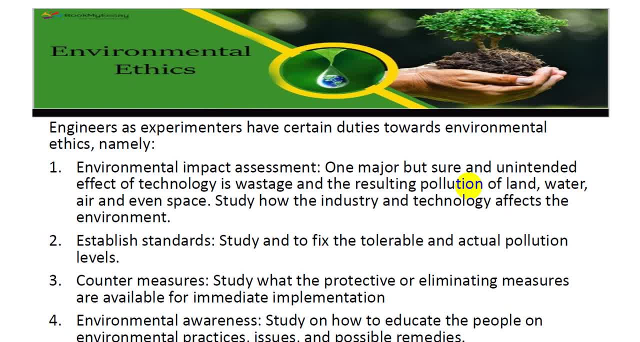 environmental awareness. but sitting at home, using social media as a tool, you can go for the environmental awareness study on how to educate the people on environmental practices, issues and possible remedies. okay, so, as an engineer, as experimenters, they have certain duties towards environmental ethics, so we just uh. to recap, there are four of 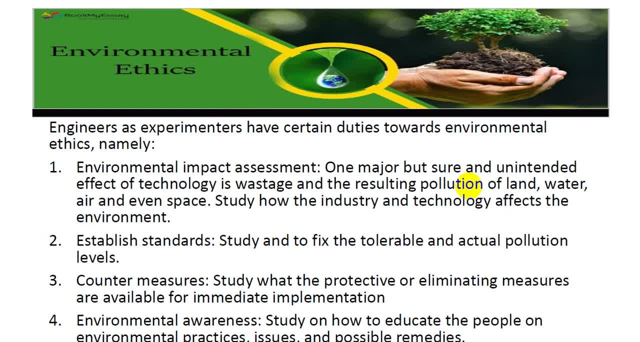 them important things: environmental impact assessment. this is number one. number two: establish standards. number three: counter measures. and number four, environmental awareness. and that is the least part. you know environment. at least you can spread the awareness. okay, so that's the lowest part, but if you do all these four, then it becomes your duty towards. 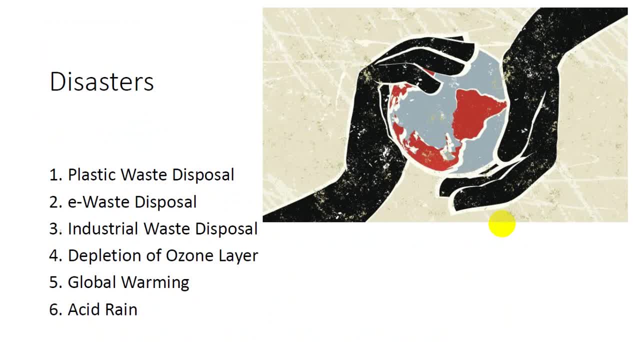 environmental ethics. okay, now, due to environment, what kind of disasters? uh, this is important. i've just, you know, gone through the internet and found these six important things to discuss today. there are the disasters that we, as humans, are causing to the planet earth. so number one is plastic waste disposal: evest what is e waste. this is important to. 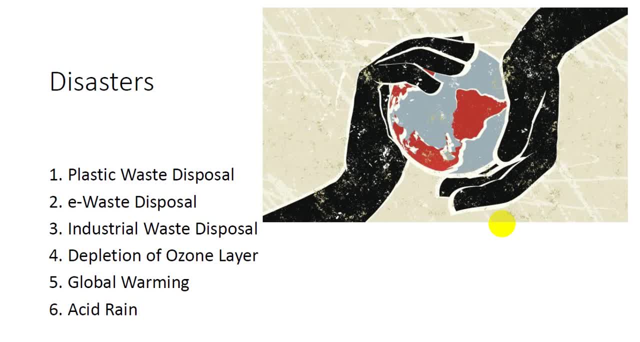 know, because now, from last 30 to 40 years, this has become one of a major problem: e-waste disposal, Industrial waste disposal. from last 100 years we are facing this Depletion of ozone layer. this is the fourth one- Global warming- and the last one is acid rain. 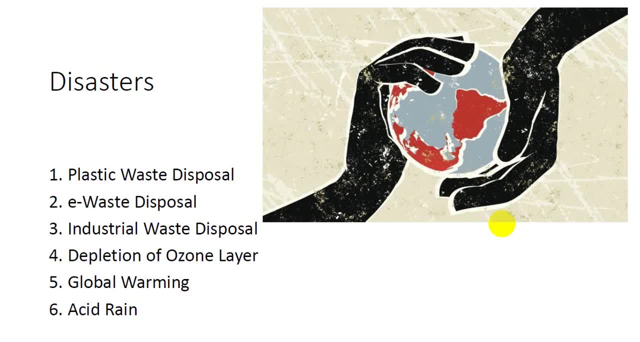 You have heard, probably from some people, from some of your friends and maybe one of your family members, about acid rain, but what it actually is and how it is formed. I have got a whole flow diagram to explain, so at the end we will just go through that. 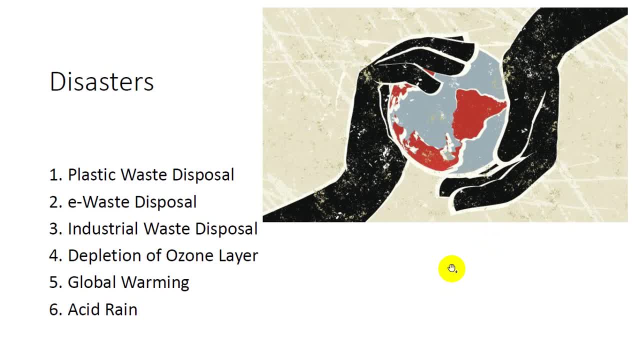 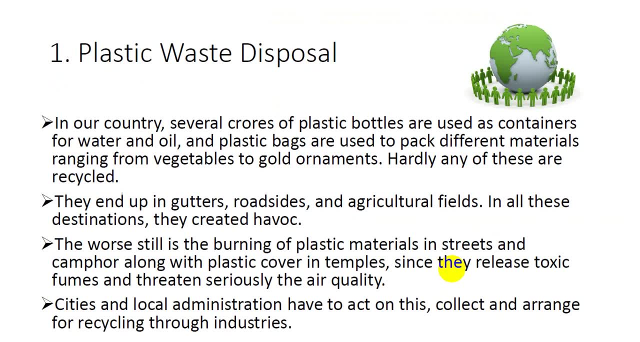 So these are the six disasters that humans have contributed to in the environment. Number one is plastic waste disposal, and this is very common, But we have started some countermeasures. As you know, now in many shops they do not give plastic bags. 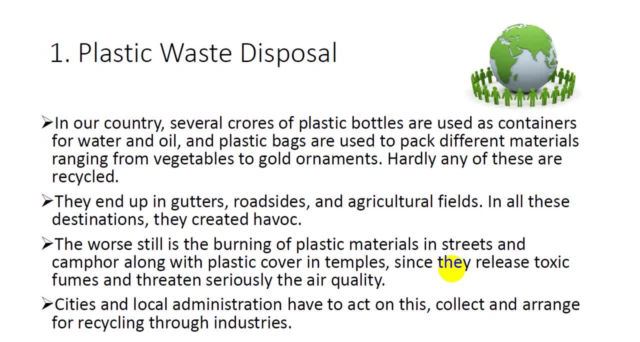 This started from Islamabad they really banned the plastic bags, And now in Lahore also this has started. And even in Comsats our director, Dr Tahir Naeem- I was talking to him- He has emphasized that from now on in Comsats and all the shops. 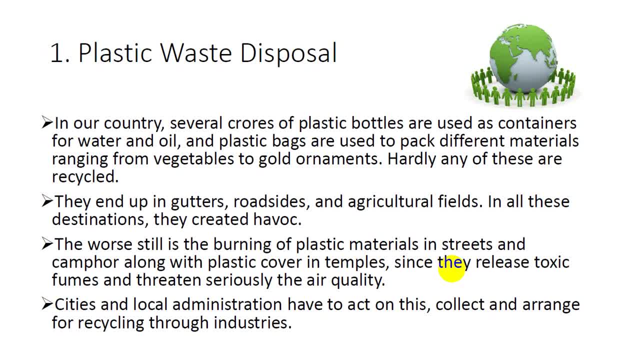 and the cafeteria, they will not sell any plastic bags, So they were going to shift the system to paper bags, Although we were always looking for much better solutions, which are you know, because anything you buy or things that you need, you know you need a bag of some sort. 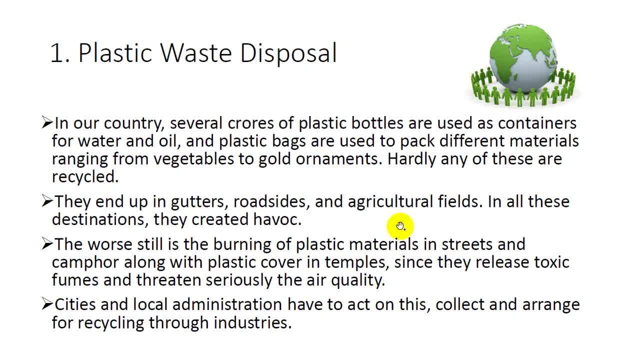 But how these plastic bags can be replaced. So this number one, the disaster part, is plastic waste disposal. in our country, Several crores of plastic bottles are used as containers. You know all the water that you drink whenever you're thirsty. 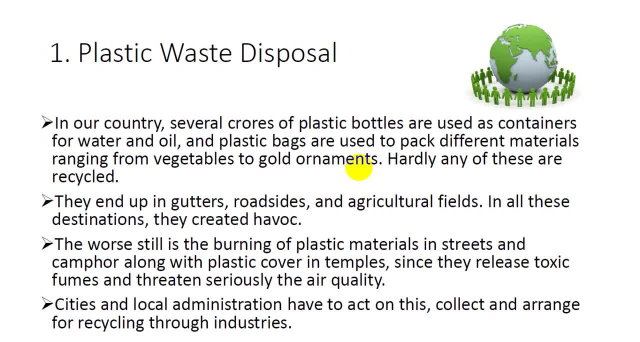 what you do? you go and buy water in what plastic bottles for water and oil and plastic bags are used to pack different materials ranging from vegetables to gold ornaments. Hardly any of these are recycled and they're just thrown into the ground phone, just like last year when we visited. 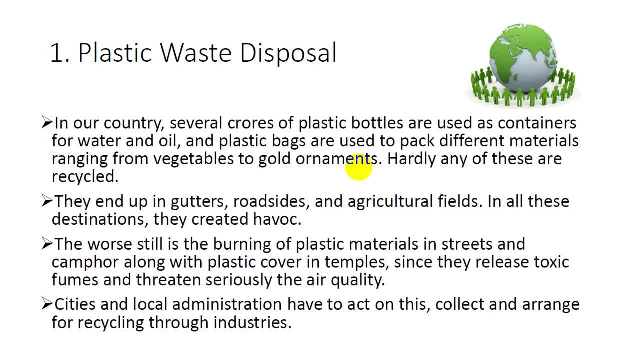 The defense wrote in for the gate in front of our main gate And we were just amazed to see so many plastic bags and cups and glasses you know all thrown into those sewage- What would you call rain drains- And they were like choked up because of this plastic disaster. 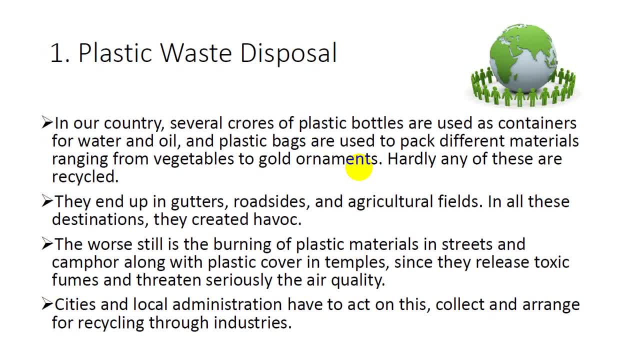 So this is one of a major thing, And now we are starting to think that what are we doing to our planet? And OK, the second part. they end up in gutters, just like I told you all the rain drains are choked up, blocked in front of the concert's main gate. 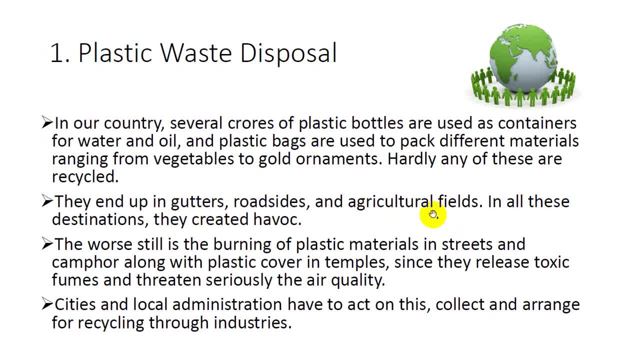 roadsides and agriculture fields. in all these destinations They create havoc. The worst still is the burning of plastic materials in the streets and camphor, And sometimes, when people don't know what to do, they just collect all the plastic. Now this is the most uneducated way of disposing of the plastic. 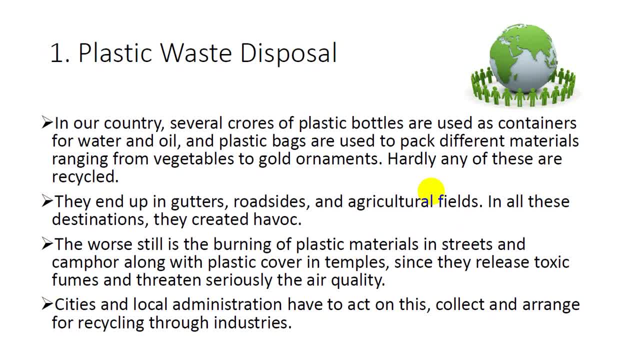 They collect all the plastic and they burn it. Now, the burning it, they're removing it from the street. But what they're doing? they're creating a really big havoc by destroying the ozone layer, Because that thing that one burns, it goes into the air and you think now it doesn't exist, but it becomes a part of the invisible air. 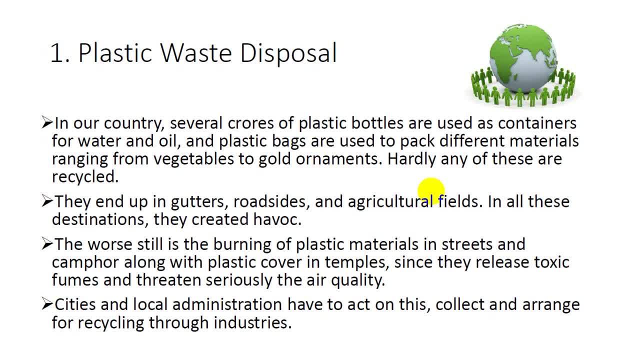 And then you start breathing that poison that before was on the roadside or some drainage. So this is the most uneducated way of cleaning, You know, when people start burning plastic materials. so what still is the burning of plastic materials in streets and camphor, along with the plastic cover in temples, since they 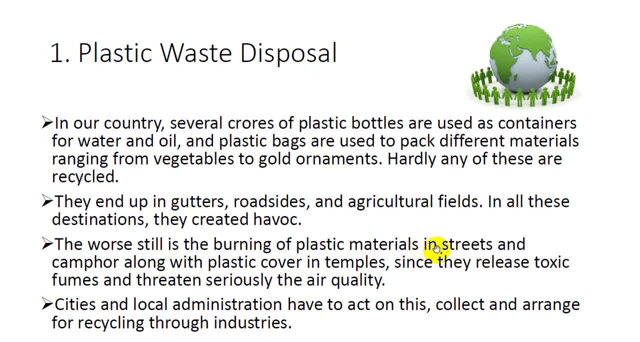 realize toxic fumes and threaten seriously the air quality. Cities and local airlines have to act on this, collect and arrange for recyclable through industry. So this is what really they need to do. This is the job of the government and also the people, the industries. 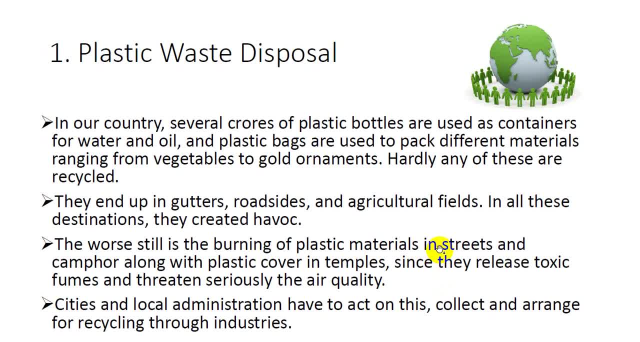 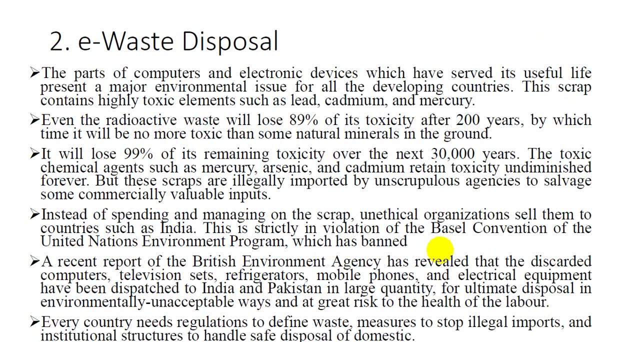 That Whenever, whenever, if they're using any plastic material, they, instead of throwing it out, they should put it in special recycled dustbins where it can be collected and recycled. okay, so this is one thing. the second is e-waste disposal. the parts of this has, you know, become a major issue. 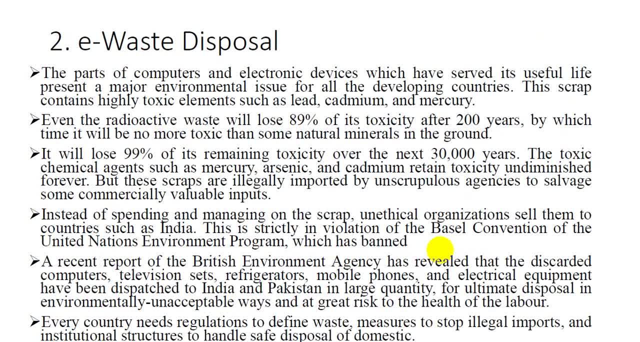 since last 30 to 40 years. before that it wasn't a big issue, but now you know, every household has a mobile phone as a computer, as cds, as you know, mouse and so many accessories, headphones, so it has become a major issue. e-waste disposal, the parts of computers and electronic devices. 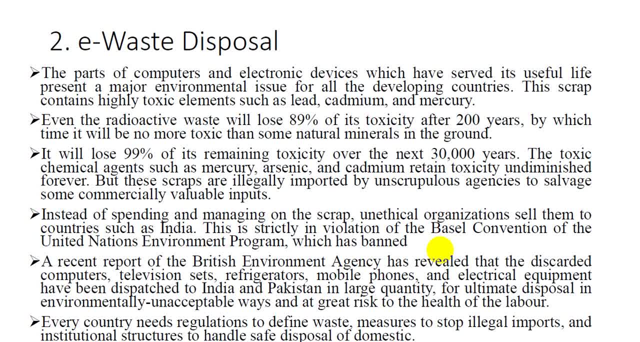 which have served its useful life present a major environmental issue for all the developing countries. this crap contains highly toxic elements such as lead, cadmium and mercury. you now you've all studied chemistry right in your fse. you know how dangerous these three are. these three can lead to cancer, and that's now, that's how, why we have so many cancer patients nowadays. 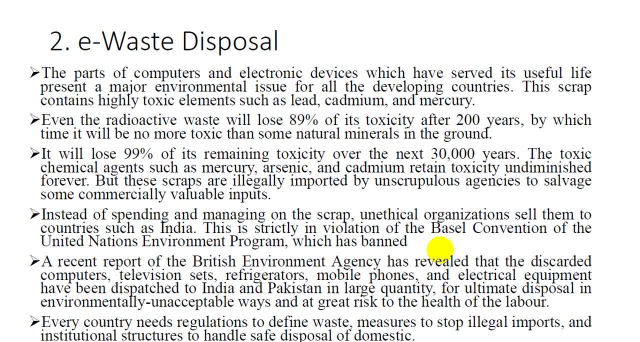 as compared to before. so lead, cadmium and mercury, this is what they add up into the our environment, into our environment, where we breathe, where we live, where we uh get food from. so if it goes in the into the soil and we're uh uh growing in, 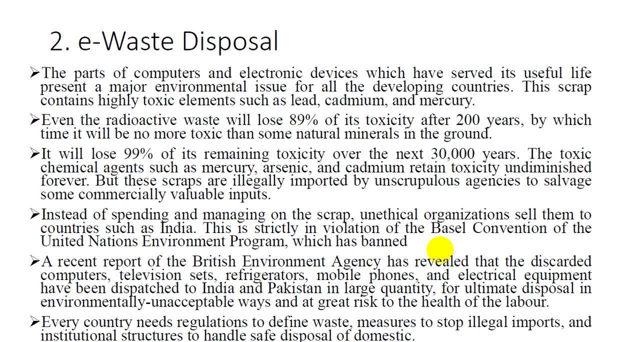 in our agriculture soil and we're growing food from there. it gets mixed into our vegetables and fruits, what we're eating, what we're breathing- everything is being destroyed. even the radioactive waste will lose 89 percent of its toxicity after 200 years. that's how long it takes. 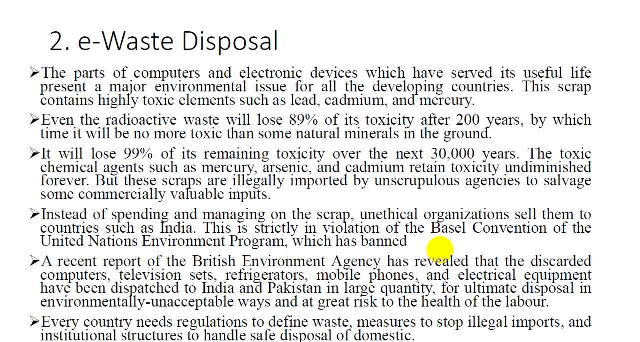 so you just put one thing now into the atmosphere. you put one thing now into the environment, into the soil. it will take 200 years to go away, by which time it will be to use no more toxic than some natural minerals. in the ground it will lose 99 of its remaining toxicity. 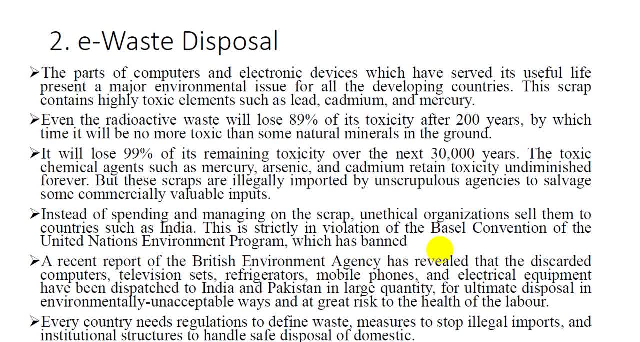 over the next 30 000 years. so 89 toxicity is reduced in 200 years and 99- nearly 99, you know, close to 100, when it's nearly all gone close to 30 000 years. so i don't know whether we'll even. 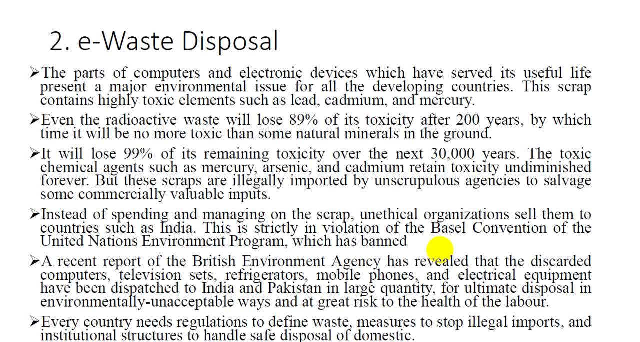 live for 30 000 years or not, but this is a hell lot of time. the toxic chemical agents such as mercury, arsenic and cadmium retain toxicity undiminished forever, but these scraps are illegal, illegally imported by uncircumcised agencies to salvage some commercially valuable. 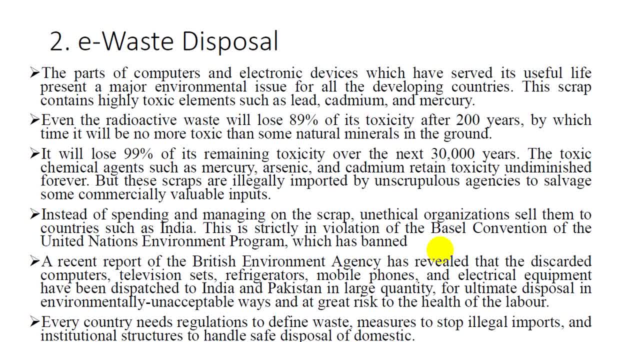 inputs instead of spending managing on this crap and ethical organizations sell them to. you can see, i have so much text in my slides, but this is. i've put all these texts. uh, knowing that you must read from here, i don't know whether you you'll probably not go and read book, although 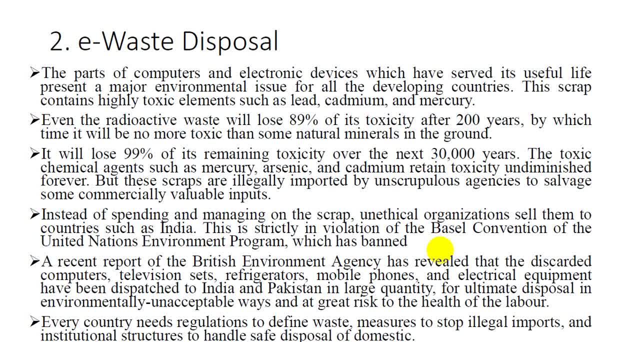 i urge you to go and search on the internet and read books related to it, but i wanted most of the text to be placed in my slides so at least you know all the facts. i just don't want to just look at uh simple words and just try to rephrase what i'm saying. i wanted you 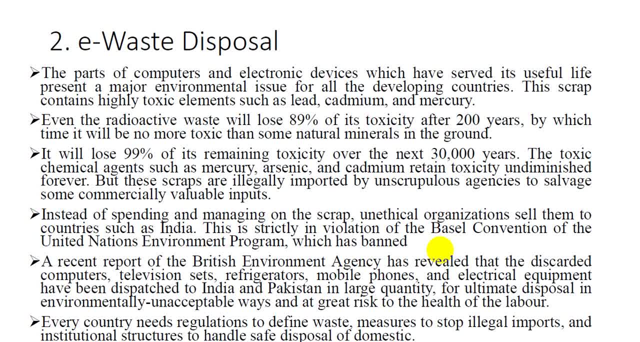 to read through all of it, just like a book. that's why i've put so much text on my slides, okay, so i want you to read through each and every sentence, okay? instead of spending and managing on the scrap, unethical organizations sell them to countries such as india, pakistan, bangladesh. 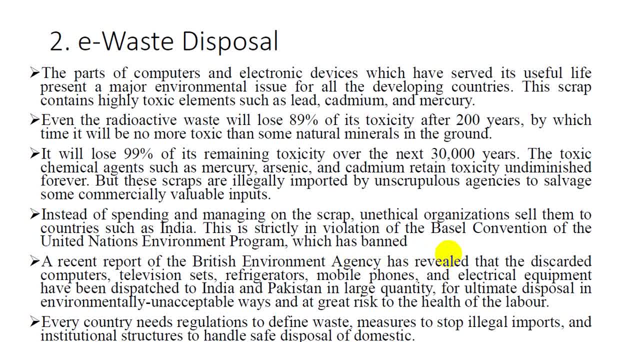 so this is what developing countries are doing: they're buying the scrap from the developed countries like england, us, europe. and what they're doing? they've become basically a graveyard for the scrap of these modern uh countries. this is strictly in violation of the basel convention of the united 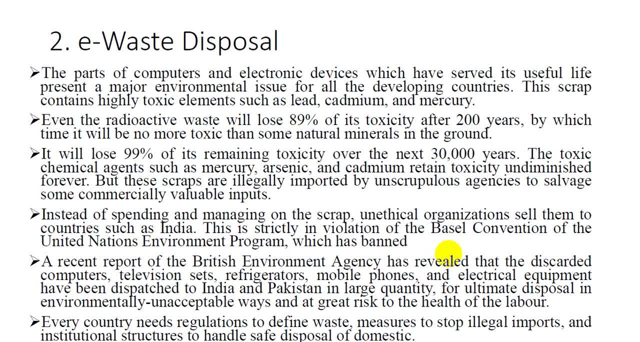 nations environment program, which has banned such activities. a recent report of the british environment agency has revealed that the discarded computers, television sets, refrigerators, mobile phones and electric equipment equipment have been dispatched to india and pakistan in large quantity for ultimate disposal in the environmentally uh unacceptable ways and at great risk to the 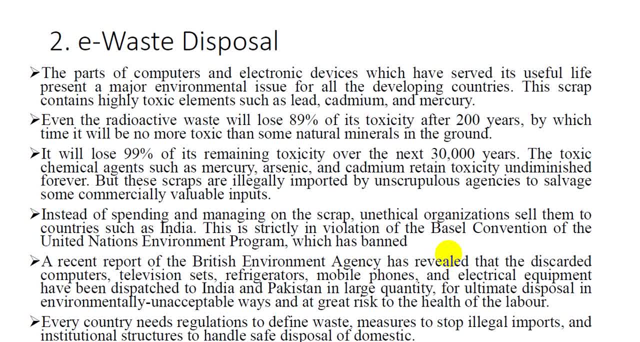 health of the labor. now what they are doing. they think, oh, recycling, oh, how do we dispose of? we don't have any disposal ability? oh, we don't have any disposal ability, we don't have any disposal. why don't we just sell it to pakistan, india? they are the developed countries, they'll buy it cheap. 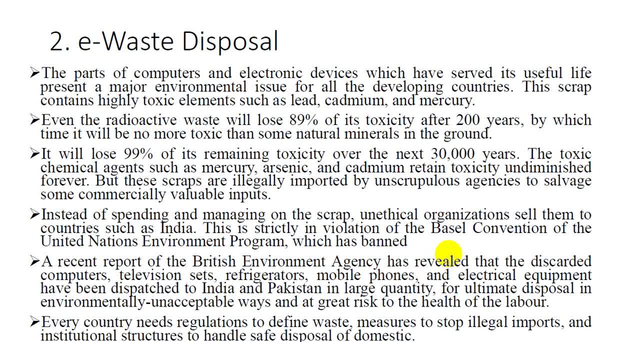 so we have become a dustbin for the europeans and the americans to sell their e-waste to us and we very, you know, very- happily just go and buy it and then bring it to pakistan and then, instead of disposing of, try to utilize some parts of it. try to some people. try to think i was really. 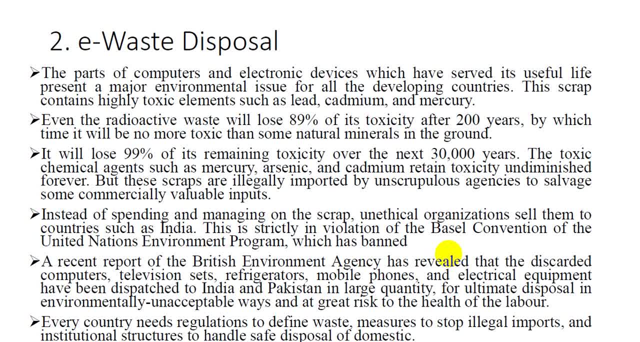 seeing this video where some people in india and pakistan what they do, that they buy it cheap- computers and laptops and mobile phones- and take out the motherboard and on motherboards, on different parts, there is some part of gold there that, as you know- your electrical engineers, you must know that some parts of lining and some uh joining some uh chips uh requires gold wiring. 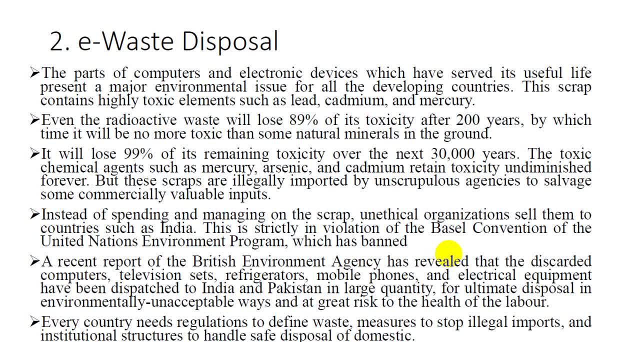 and gold etching so they melt all that plastic and all that thing and throw it in our environment just to get that little bit of that milligram of gold from the motherboard. and that's what. that has become a major business in pakistan, in india, every country. 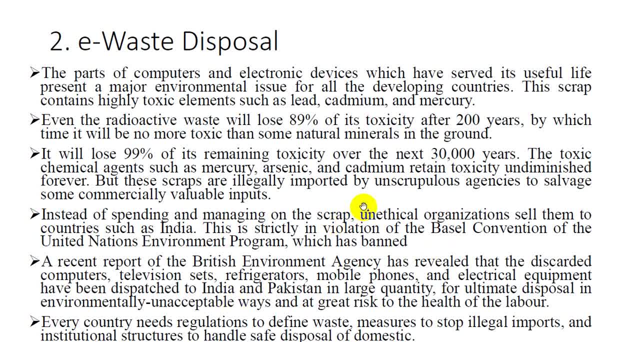 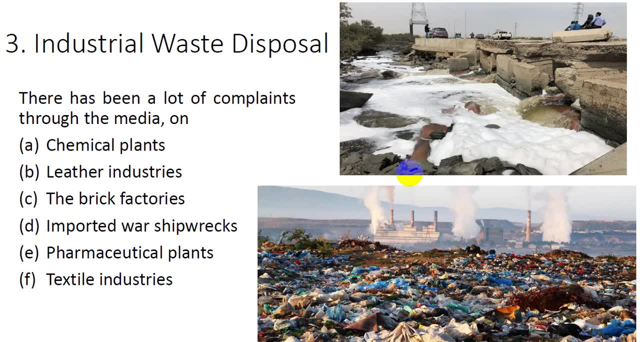 needs regulations to define waste, measures to stop illegal imports and institutional structures to handle safe disposal of domestic okay. so e disposable, e-waste disposal. this is the second disaster. the third one is industrial waste disposal. so i've taken some pictures. you know, these pictures show what our industries are doing. you know, in one on one part we want to support our 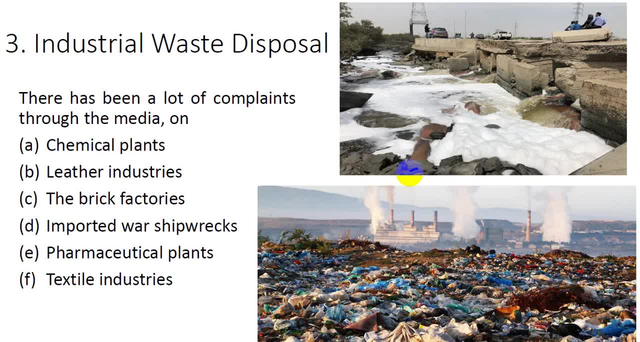 industries that whatever we want product will make it in our home and then export. but then what we are doing? we're destroying the environment because those industries are not properly regulated by the government and they don't have any plants. they don't have filter plants, so anything they make, all the, the, the chemicals. 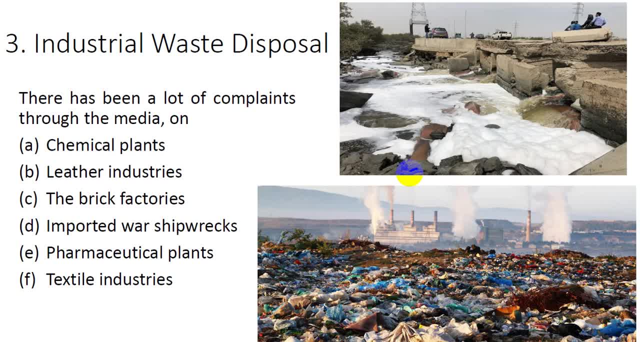 that they just dispose of in the drainage and sewage and then in the environment. there has been a lot of complaints through the media on chemical plants, leather industries, the brick factories, imported warship wrecks, pharmaceuticals plants and textile industries, although these industries are important for our future. but 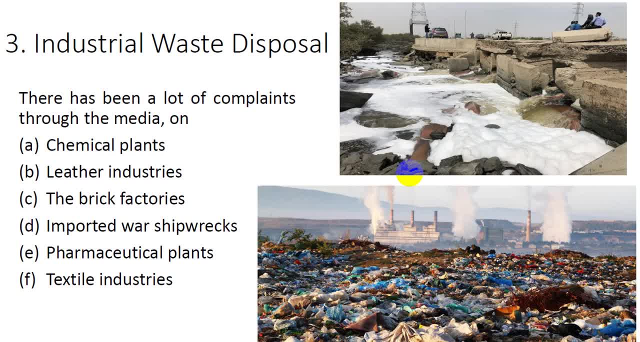 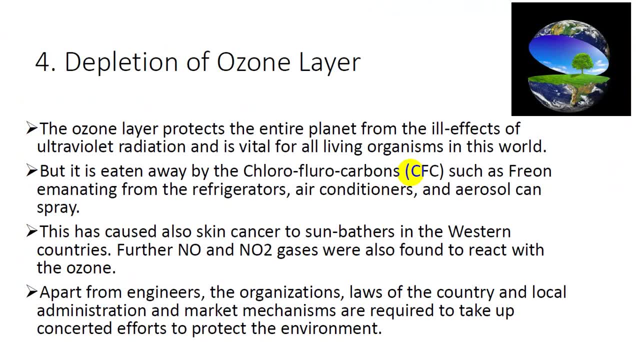 they must also have a filtration plant. this is the third one. the fourth one is depletion of ozone layer. uh, you've probably heard on tv, watched many videos. uh, the ozone layer protects the entire planet from the ill effects of the ultraviolet radiation and is vital for all living. 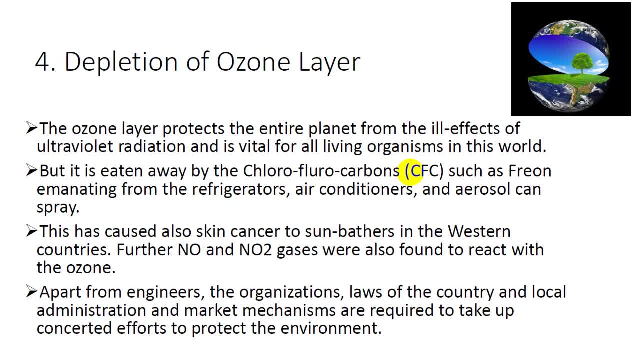 organisms in this world. so it is a cloud, it is a blanket that is protected, protecting us from the ultraviolet rays coming from the sun. if we destroy that blanket, we'll be just all burning to. you know, like burning uh. daily you walk out the ultraviolet rays would just kill you. the only 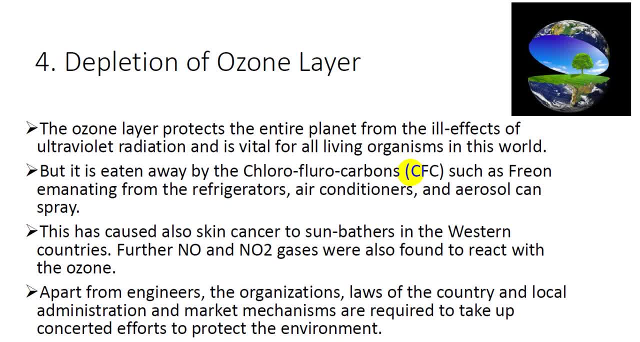 thing that is saving you is the ozone layer and what we are doing with our environment. we, we are making uh such e-waste disposal and uh plastics and all these things and we are basically destroying our own ozone layer. cold, uh and feeling the cold and has a blanket just to save him- uh, save his life- and he starts. 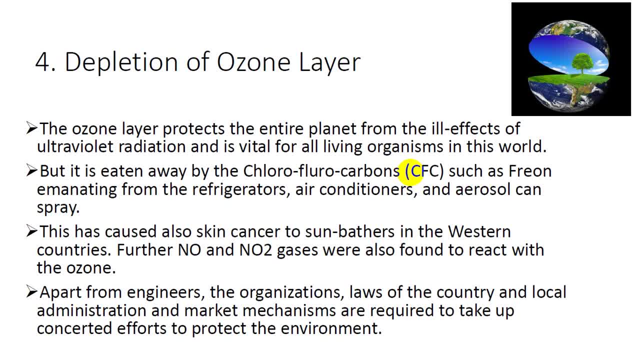 uh burning his own blanket. this is what we are doing, but it is eaten away by the chlorofluorocarbons, cfc, such as freon, emanating from the refrigerators, air conditioners and arsenal. uh aerosol can spray, can spray. so these these things have a cfc which basically uh eats up those. 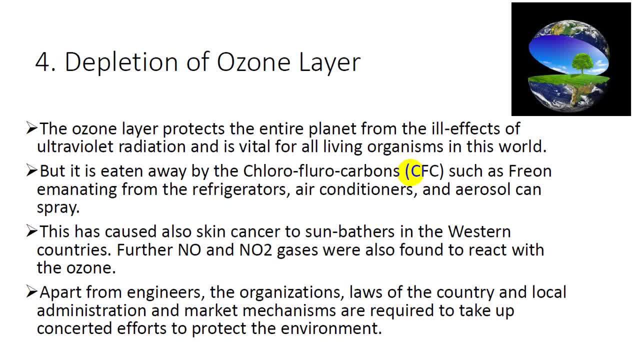 but now the new, what? engineers are, of course, contributing in some part. so what they have done, that now the new inverter air conditions that are coming, they have much better gas, they have a safe gas. so even if there is some leakage, it doesn't uh, it's an environmental environment. 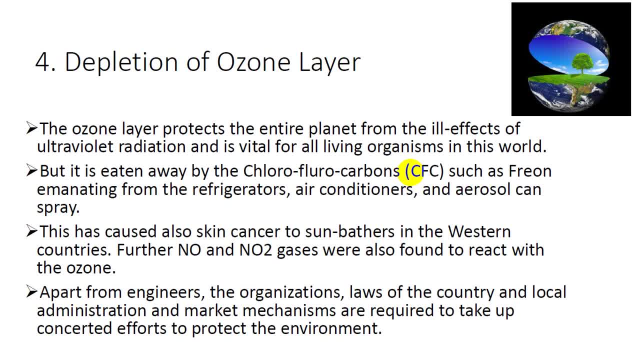 safe gas and it doesn't uh eats up the ozone layer. so these are some of the things that we are doing now. this has caused also skin cancer to sun bathers in the western countries. further uh oxygen oxide gases were also found to react with the ozone. apart from engineers, the 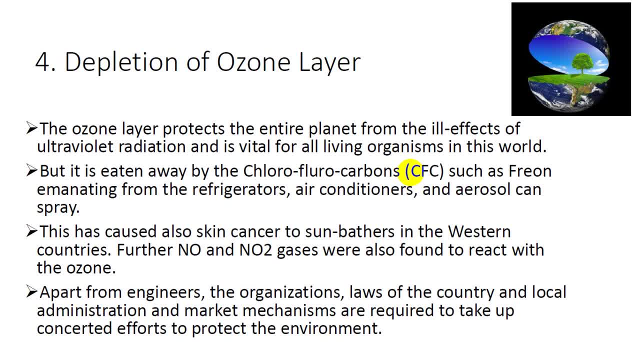 organization's laws of the countries and local administrations and markets mechanisms are required to take up the concerted efforts to protect the environment. so these are some of the gases that, whatever we design, whatever- even if you're designing the air conditioners or other refrigerators- we need to design them and use gases that are environment friendly and that do not. 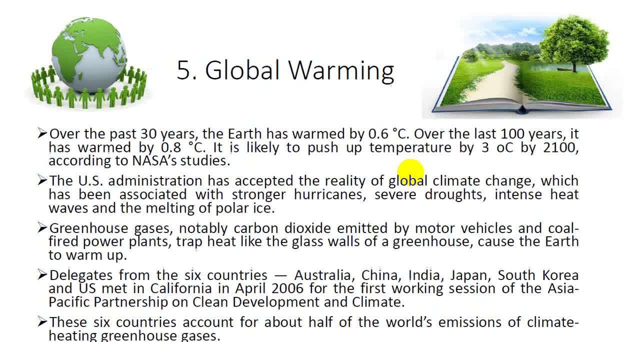 affect the environment. so these are some of the things that we need to do to protect the environment. okay, the fifth one is global warming: uh, over the past 30 years, the earth has warmed uh by 0.6 uh degree degree centigrade. over the last 100 years, it has warmed by 0.8 centimeters, so 0.2. 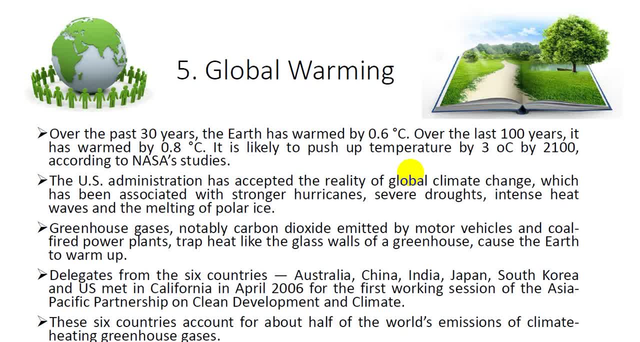 degrees centigrade. it has increased. it is likely to push up temperature by 3 degrees centigrade by 2100. so it's going, you know like. exponentially it's rising, according to nasa's studies. the us administration has accepted the reality of global climate change which has been associated. 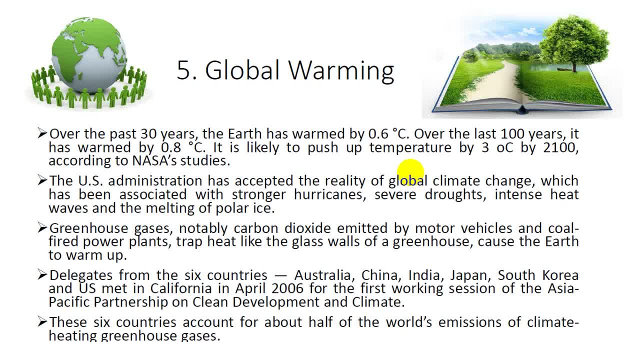 with stronger hurricanes, severe droughts, intense heat waves and the melting of polar ice. greenhouse gases, notably carbon dioxide, emitted by motor vehicles and coal fire plants trap heat like the gas glass walls of greenhouse, cause the earth to warm up. delegates from the six countries australia, china, india, japan, south korea and us met in california in april 2006. 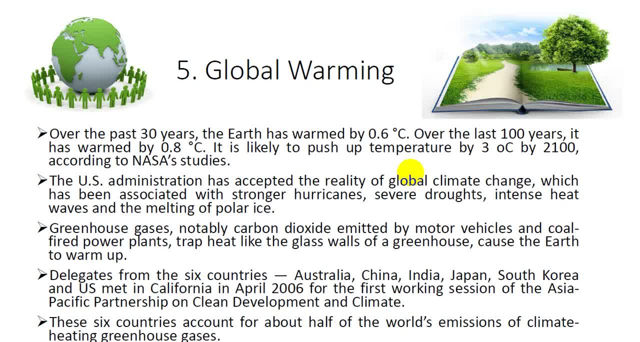 for the first working session of the asia pacific partnership on clean development and climate. these six countries account for about half of the world's emission of climate heating greenhouse gases. so global warming is related to the emissions of climate heating greenhouse gases. so when you see that you know, uh, these hurricanes and these floods, they, they didn't used to exist. 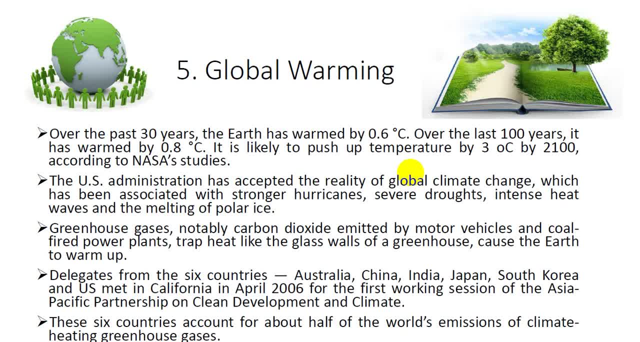 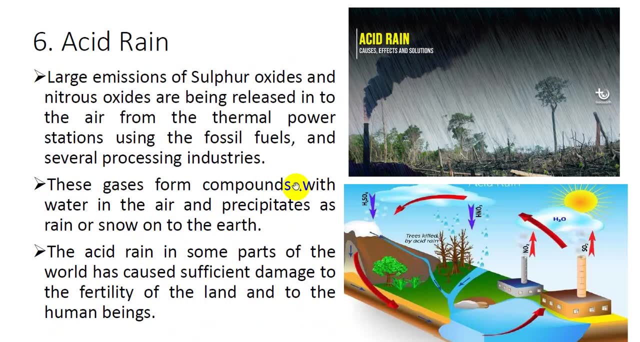 about 20, 30 years ago, or they should be very rare. now it's just like every year. why is it happening? because of global warming. so you must realize how uh human beings are uh tarnishing the planet earth. okay, this is the. now the last one, the sixth one. i told you in the beginning. i will tell you the whole. 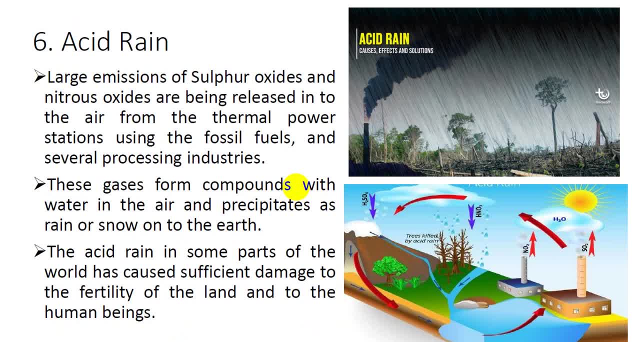 flow of the acid green, how we produce, uh, how the acid rain is produced. so what happens is that large emissions of sulfur oxide and nitrous oxides are being released into the air from the thermal power stations. okay, using the fossil fuels and several processing industries, you can see the uh the this diagram. 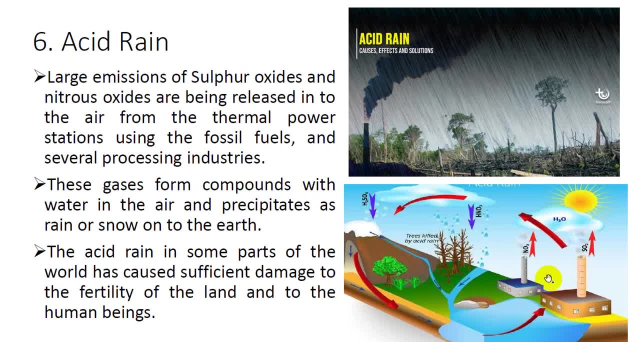 at the bottom uh, bottom right uh corner how sulfur oxide and knife nitrogen oxide goes into the air, mixes with h2o. these gases form compounds with water in the air and precipitates as rain or snow on the earth, so it becomes hno3. okay, the acid rain in some parts of the world has caused 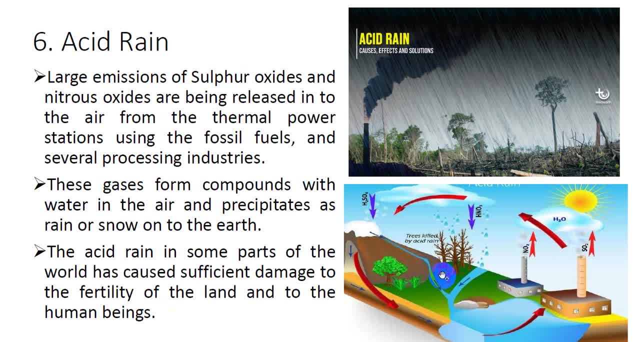 damage to the fertility of the land and to the human being. so you say, this land used to be very green and we were growing crops, and now nothing's happening. where did this drought came from? it came from your industry, because you were burning the sulfur oxide and nitrogen oxide into the air. 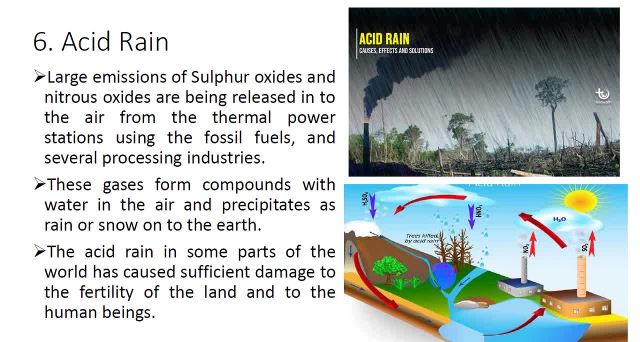 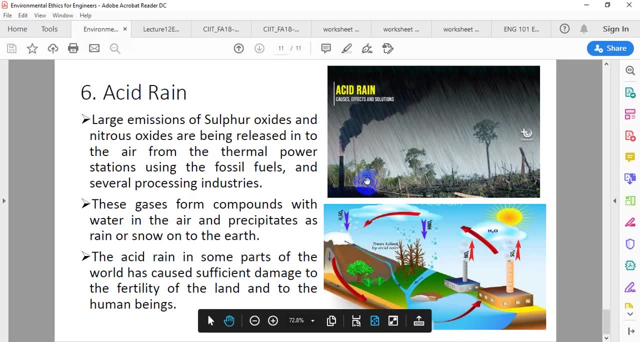 and it produced acid rains which destroyed your crops and your land. so this is also an important part. so these were the six disasters, uh that we were talking um. this next lecture, we'll be talking about the sustainability, the sustainable development. so in today's lecture, it was all about, uh, environmental ethics for engineers, uh. in. 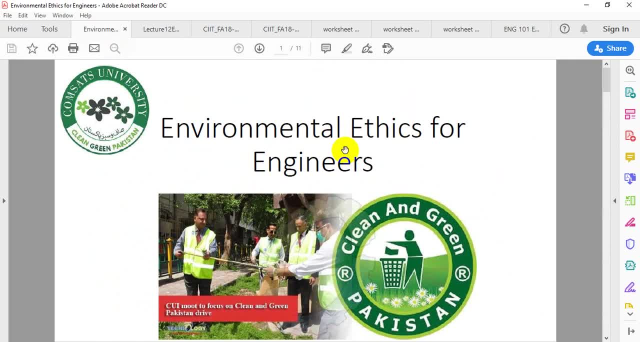 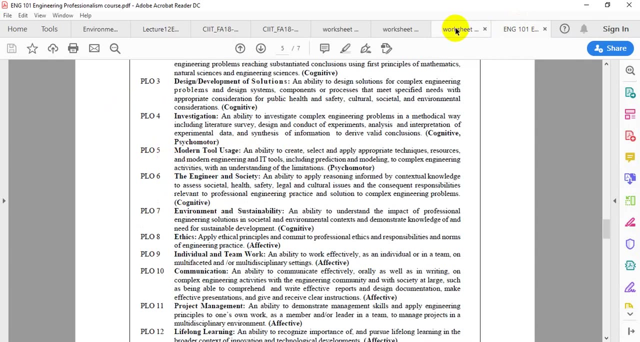 next lecture, which is tomorrow. uh, you can listen to my lecture regarding sustainable development. that is also very important and in that lecture, we'll be talking about the ecology, the economics and, you know, many other things related to the sustainable development, like human-centered ethics, uh, sentient-centered ethics, environment-centered ethics. so, and what? 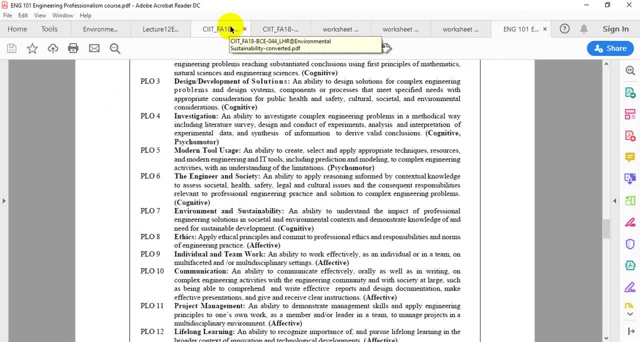 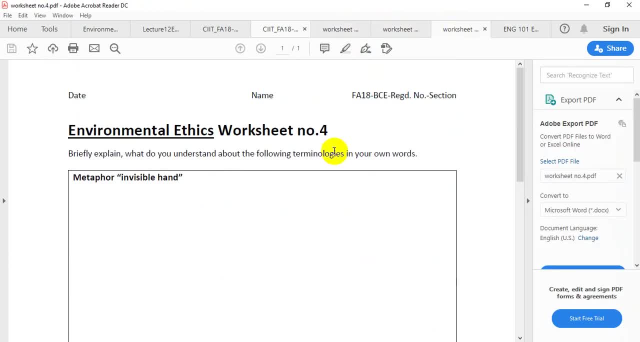 is sustainability and what is sustainable development and how. what roles engineers play in that? okay, so, uh, before we go, uh, there, i want you to, i want to give you a brief homework, so i want you to briefly explain: what do you understand about the following terminologies in your own words: you: 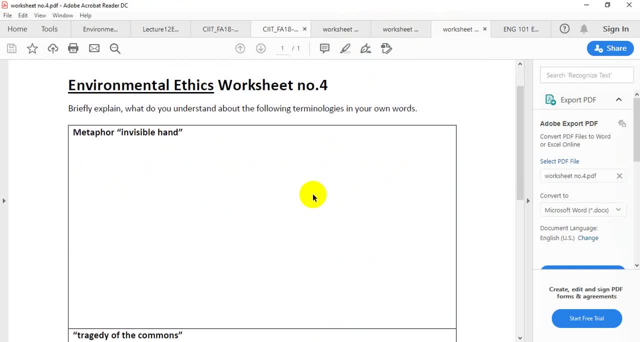 know what? uh, there are two main terminologies in your own words. you know what? uh, there are two main metaphors. uh, we would be discussing them in the next lecture, but i want you to just initially, before we start tomorrow's lecture, know what do we mean by search on the internet. 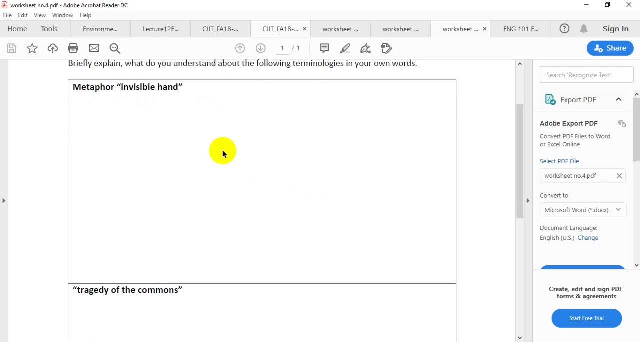 search on the go and read the book. you can search on the book in the environment and sustainability chapter. what do we mean by invisible hand and tragedy of the comments? okay, so this is your, just your homework that i want you to do. this is worksheet number four.